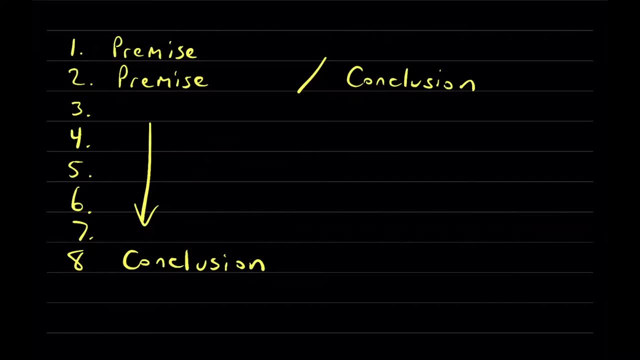 One or more premises And then you have a conclusion that you're trying to demonstrate follows from those premises. So what I've done here is I've enumerated, you know, this argument would have two premises and a conclusion. What you're trying to do, in a series of steps, is to demonstrate that the conclusion follows from those premises, as indicated by the arrow here, from a series of steps, using 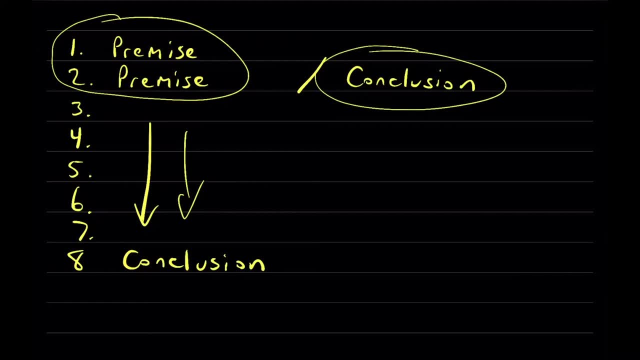 valid inference rules and valid rules that dictate what types of statements follow from statements that are given to you in the argument. So all Proofs look like this: You start out with a couple of premises that are, you know, the premises of the argument, You're given some conclusion you're supposed to demonstrate And then you deduce further things that have to be true. 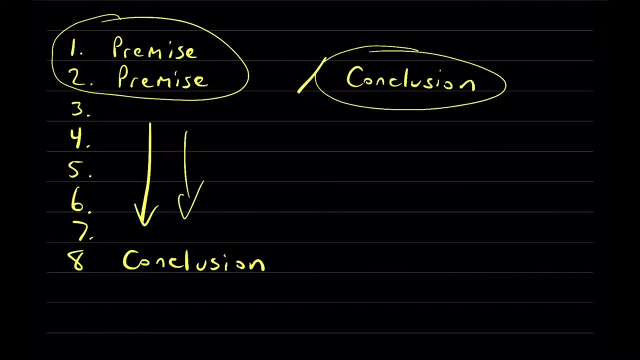 Given those premises, given these logical deduction rules that you're going to learn- And there are a bunch of these- We're going to learn four of them today. We're going to learn a fairly large number of these over the next several weeks. All of these I should mention are inside the inside cover of your textbook, And feel free to use that when doing your homework. You should. 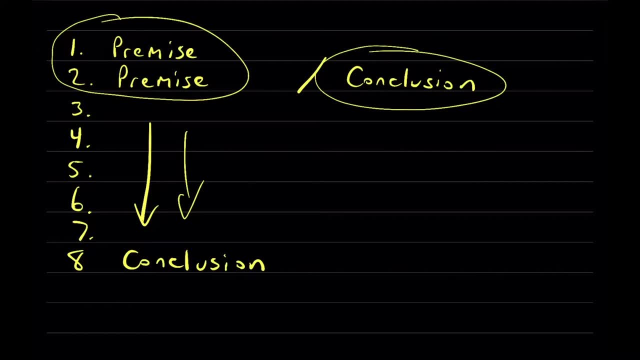 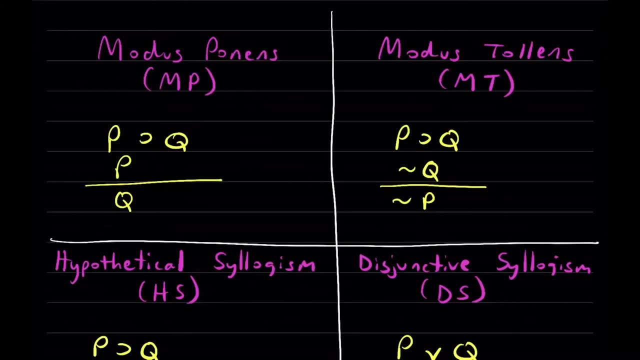 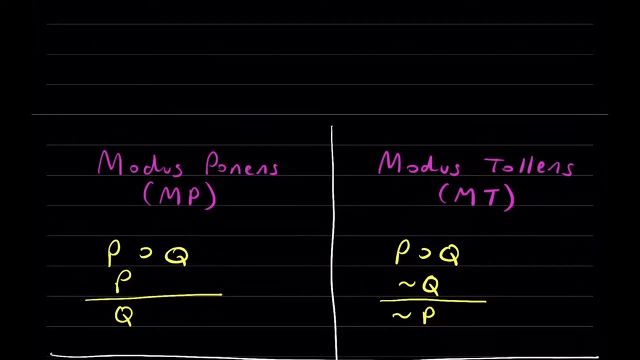 It would be almost impossible to do proofs without something like that handy. There's more I could say here, but I think I just want to dive in and start introducing these deduction rules. These deduction rules are fairly intuitive, In fact, like I said, natural. the whole point of natural deduction is that they mirror the way we use reasoning in ordinary language. 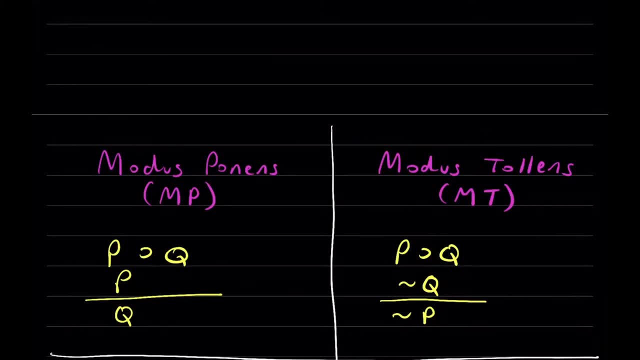 You'll have to kind of forgive these, these Latin names for these rules. These are the canonical names for these rules And unfortunately a couple of them are not. A couple of them are fairly easy to confuse with each other, like these two here: modus ponens and modus tollens. Fairly easy to confuse those with each other. Let's go ahead and dive in. 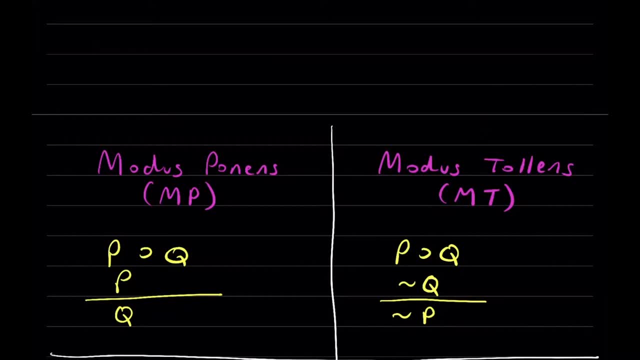 If you're given an argument like this, where you have if P implies Q right here, That says that if P is the case, then Q is the case. That's what an if-then statement means. If you then know that that P is actually true, the antecedent of that conditional, you can deduce that Q follows from that. 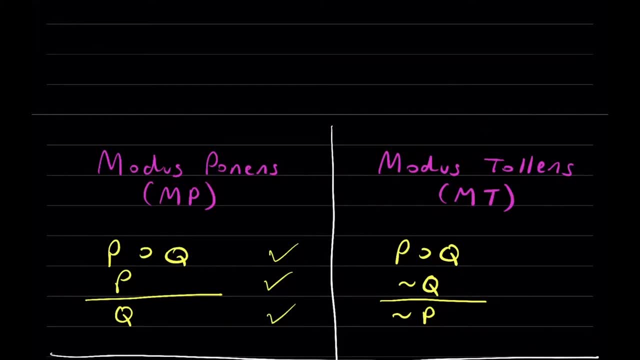 And this is probably the easiest inference rule to understand, right, If you have a statement like if P then Q, and you know P is true, you know from that that Q has to be true. So that one's pretty straightforward. I should say as well that P and Q here are just placeholders for any statement, either a simple statement or a complex statement. So for modus ponens you could have something like: if A then B, A therefore B. 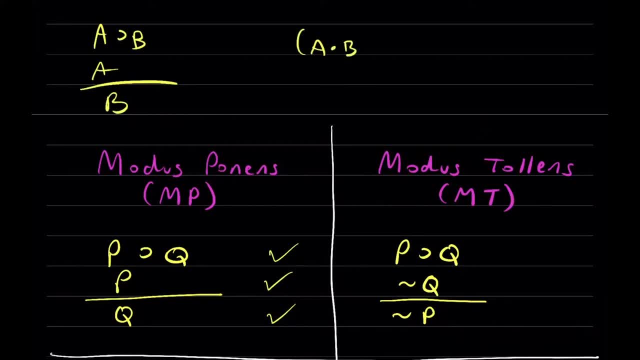 But you could also have something like this: If A and B, then C and D. That's a conditional as well. So here A and B would stand for P and C and D would stand for Q. If you then know that A and B are actually true on a separate line of the proof, you can conclude from that that C and D are true as well. 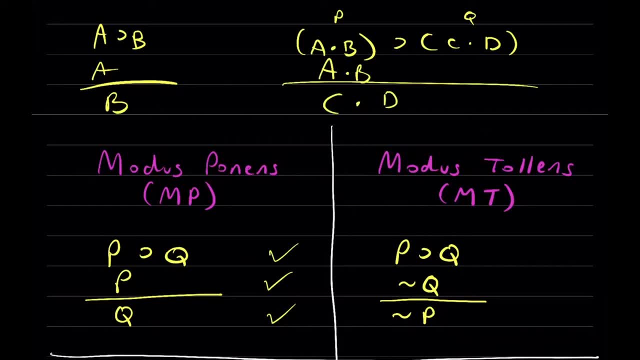 So again, this argument has that same pattern. If P, then Q, this is P therefore Q. So any argument that has that pattern, no matter what you plug in for P and Q, whether a simple statement or a compound statement, Q would follow from those premises. Again, whether P or Q are simple or compound, 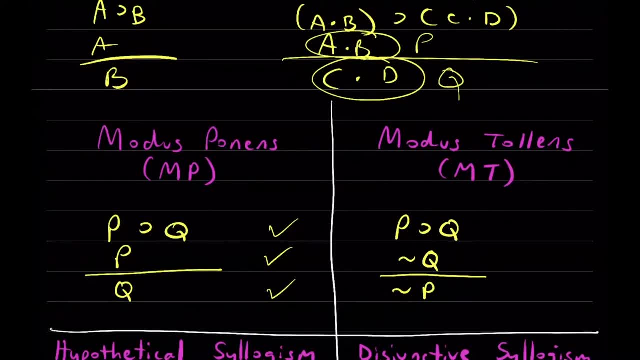 Let's talk about modus tollens. Modus tollens also has a conditional statement: if P, then Q. But in this case you have the negation of the consequent, not Q, And if you know that Q is false, then that means P has to be false as well. 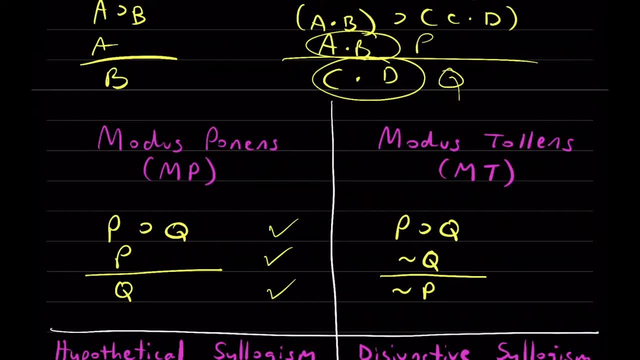 And I think this is a little harder to understand, but not much harder to understand. If P were true, Q would have to be true. That's what the first premise tells us. But if we know if Q is false, we know from that that P has to be false. 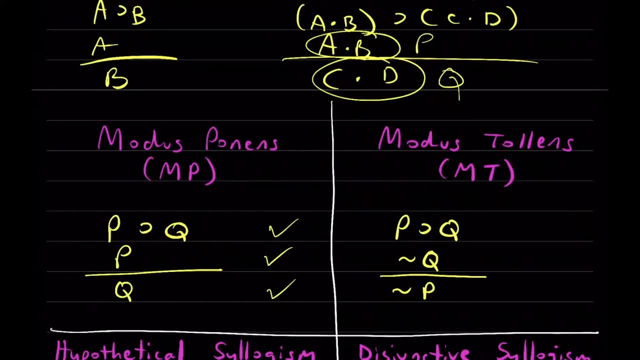 So, again, the way modus tollens works is that you always have a conditional and you have a negation of the consequent and you can conclude from that the negation of the antecedent. If you think about what those premises are really saying, you should be able to tell why that argument is valid. 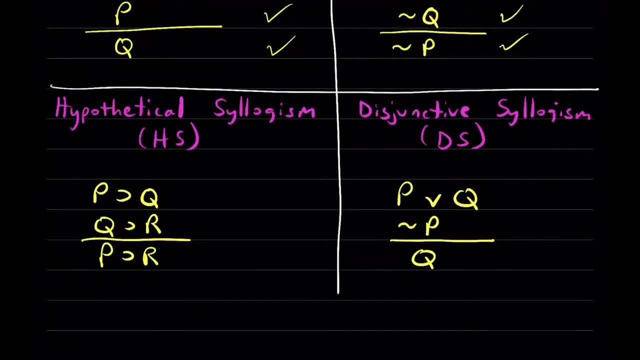 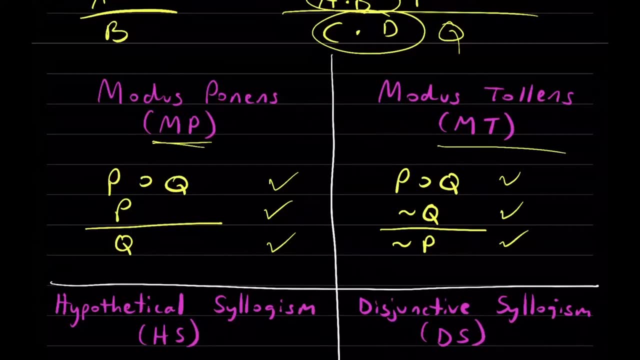 The next inference form is hypothetical syllogism. Oh, I should say as well that it's common in a proof to abbreviate these inference rules. It's the same way but with different syllables: Modus ponens would be M-P, modus tollens would be M-T. 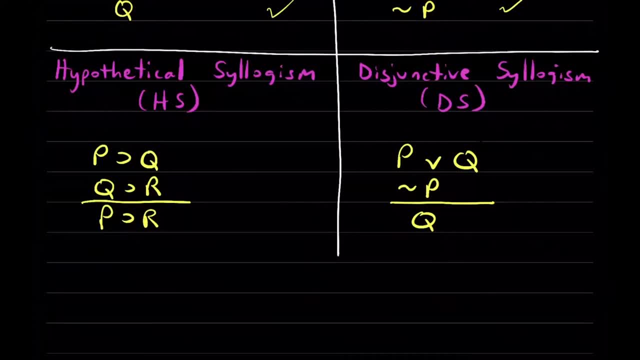 The next rule I want to look at is called hypothetical syllogism. Your textbook calls it pure hypothetical syllogism. A hypothetical syllogism always looks like this: you have a conditional- if P, then Q, and the consequent of that conditional, Q, is the antecedent of another conditional. in this case, Q implies R. 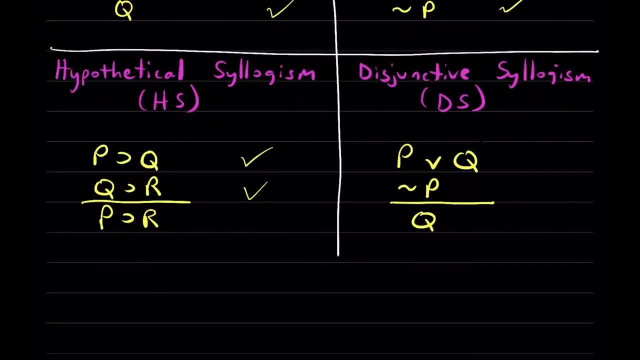 And I think, implies Q, but Q in turn implies R. that means that P would have to imply R, If P then Q, but if Q then R. so if P then R. Hence the conclusion there: if P then R. And the last rule: we're going to look. 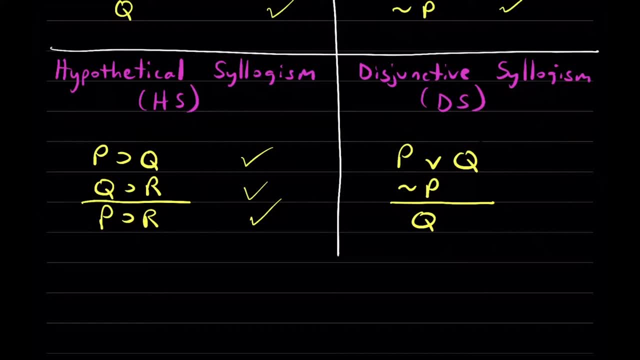 at today is called disjunctive syllogism And, if you remember, a disjunct is an either-or statement, as symbolized by the wedge in that first premise. So the first premise is not an if-then statement, it's a disjunction either-or statement, either P or Q. And if either P or Q is true, and you know, 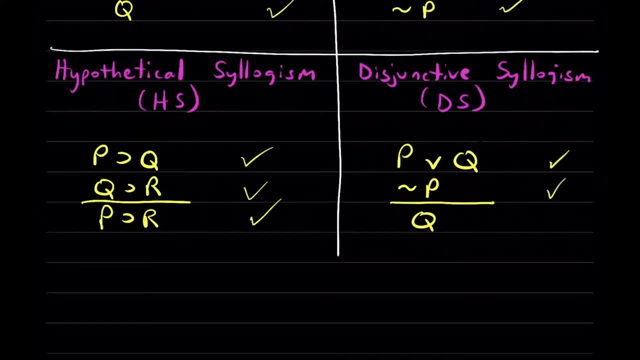 one of them is false, in this case P. you know that Q has to be true, And this is exactly how we use an either-or statement If either P or Q has to be true. but we know P is false, Q would. 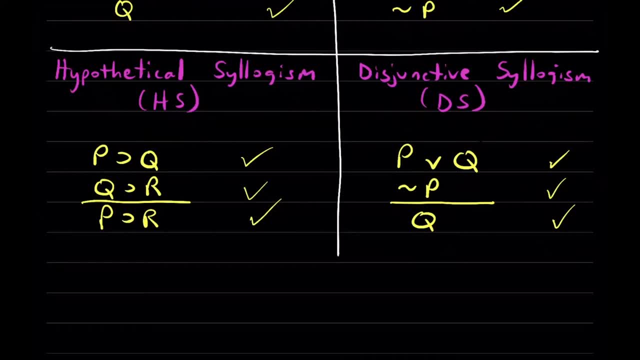 have to be true. It is important to notice that for disjunctive syllogism you technically have to have the negation only of the term on the left. Now, obviously, P or Q and Q or P mean the same exact thing. 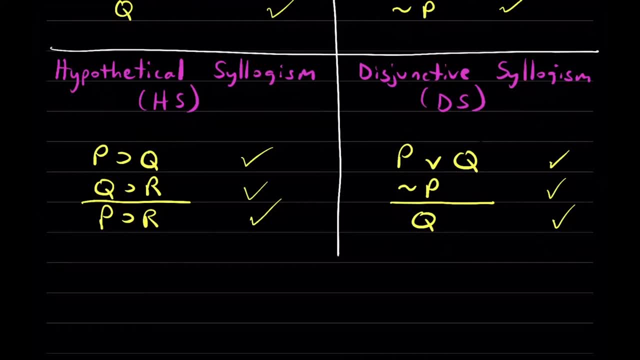 But you're going to learn another rule in a couple of weeks that lets you switch around the order of a disjunction. You don't have that rule yet. So basically, a disjunctive syllogism always has to have the negation of the term on the left, in this case the negation of P. So that's a disjunctive. 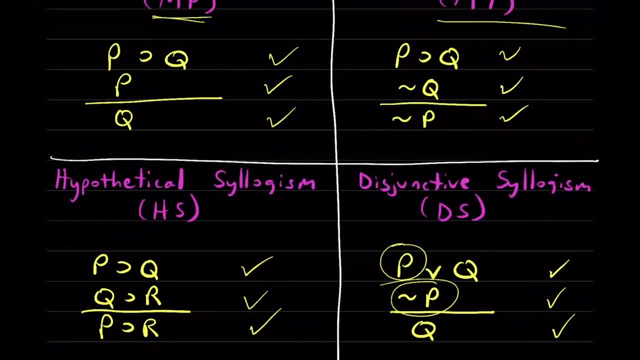 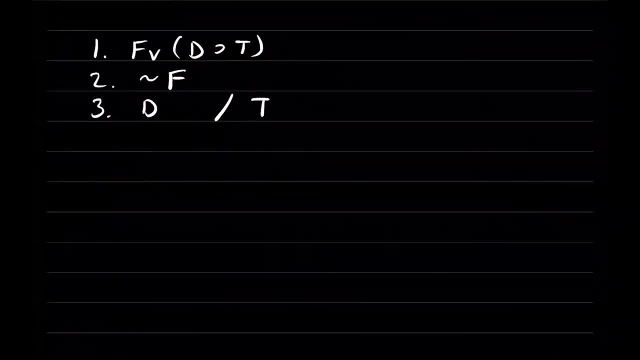 syllogism. These are probably the four easiest rules of everything you're going to learn when doing a proof. And again, don't let proofs become too overwhelming. They are really intuitive. In fact, they're way more fun, honestly, than doing truth tables. Truth tables can get unwieldy. 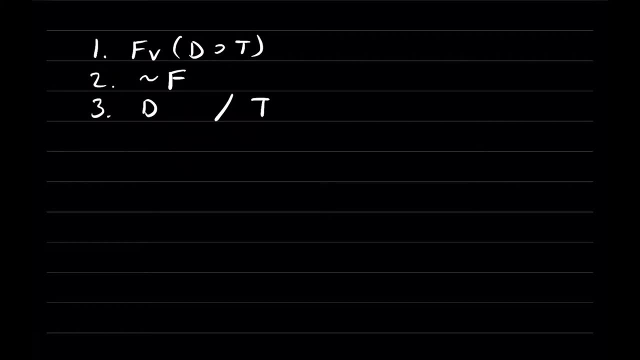 really quickly. I think you can see that as arguments get larger, with more and more simple terms in them, truth tables are going to get massively unwieldy. An argument with only a single letter would only have two rows, But if an argument has two letters, it'll have four rows, If three letters it'll be. 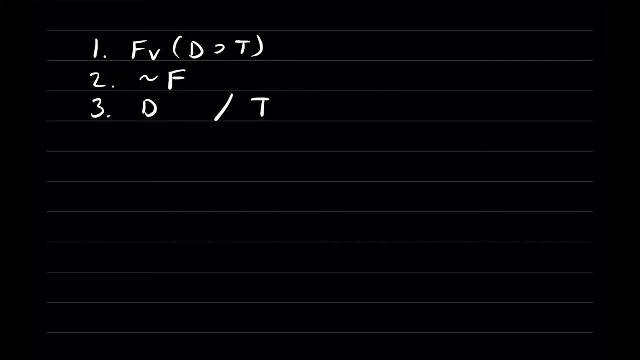 eight rows And you can see that that's exponential. So, before you know it, you're doing truth tables that have 16 rows, or 32 rows, or 64 rows, or 128 rows, or even 512 rows or 1,024 rows. That is so. 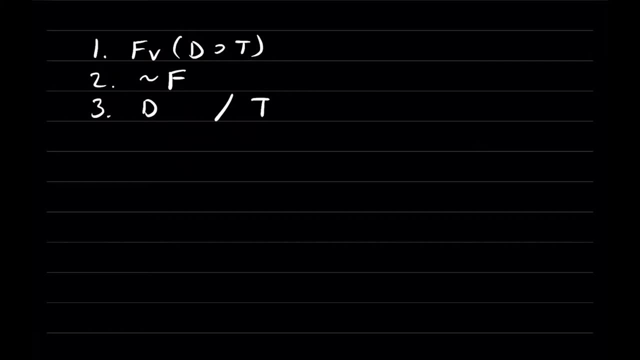 massive. you can't even fit it on the side of a building. You know pretty soon you won't be able to fit it on the side of a skyscraper. So it's not a very extensible method for showing that arguments are valid or invalid. Proofs are a much more elegant way of showing that arguments are. 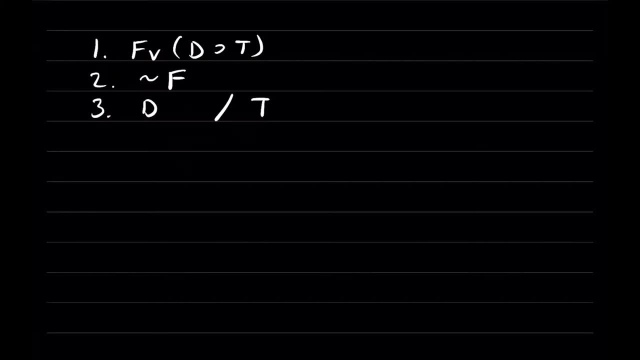 valid. All of the challenge in doing a proof is in pattern recognition. You have to be able to look at these, the statements, and make up an argument and identify the patterns of those inference rules inside the statements of these arguments, And that just takes practice. So from here on out, 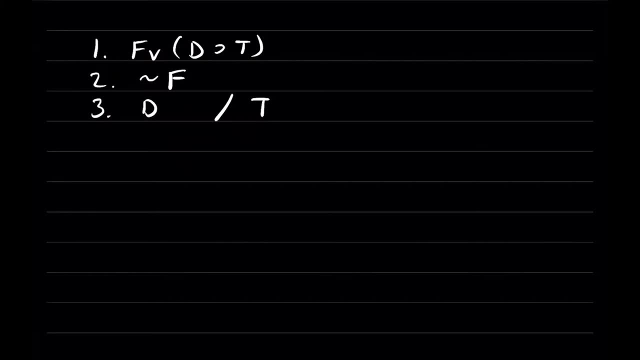 for the rest of this video, I'm going to show you how to do it. And I'm going to show you how to do it. I'm going to do example after example after example of proofs showing how to identify the patterns of those argument forms that we looked at just a moment ago, and just sort of. 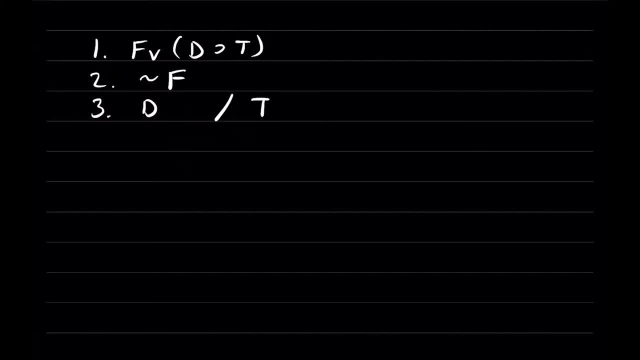 teach you by example how to do proofs. I think you'll see this is a lot more elegant than doing a truth table. In fact, if we did a truth table for this argument, there are three simple statements here. This truth table for this argument would have eight rows and we're going to be able to. 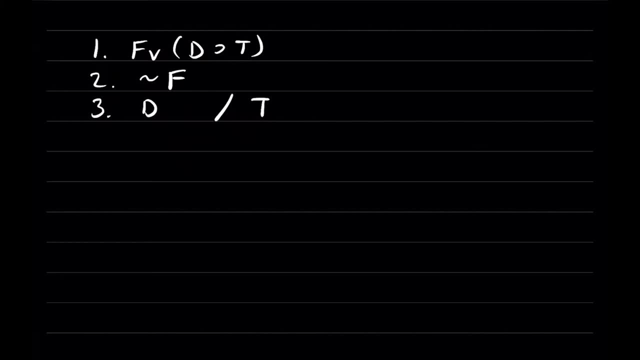 do a proof for this argument very, very quickly. So this argument: we're given three premises. Premise number one is F or D implies T, The main operator. there would be a wedge. Make sure you notice that The second premise is just not F, so we know F is false. And the third premise: 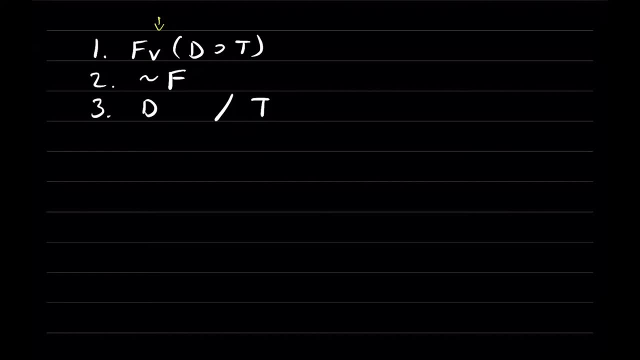 D tells us that D is true And we're trying to prove the conclusion. So the first thing you want to do when you're doing a proof is make sure you look at the conclusion, because that's how we're going to know. when we're done, We're going to start deducing further statements that have to. 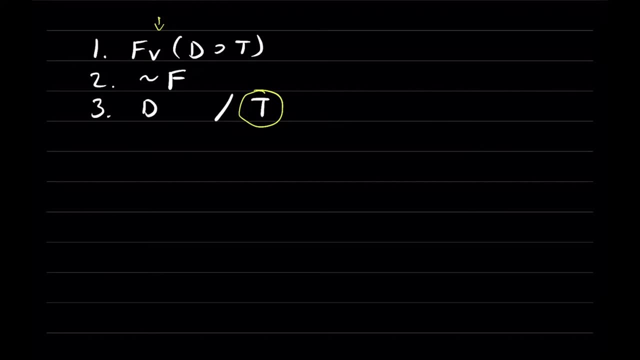 be true. given the truth of these premises, And as soon as we can get T on its own, we're going to add a new line of the proof. we're done and we've shown that T necessarily follows from those premises. I'm just going to dive in. So we're going to add a new line, number four, And there's 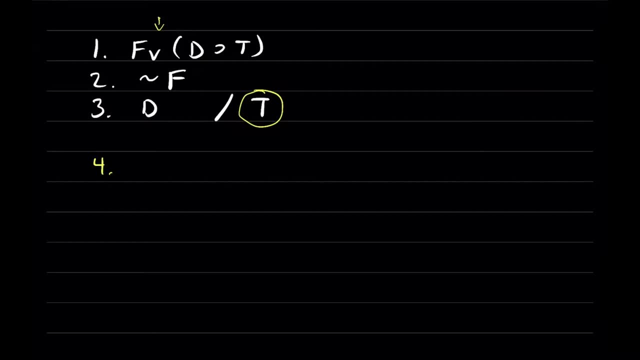 only one starting place here, given the rules that we have. Premise number one tells us that either F is true or everything in those parentheses is true. But the second premise tells us that F is false, And that should flag you as a disjunctive syllogism. 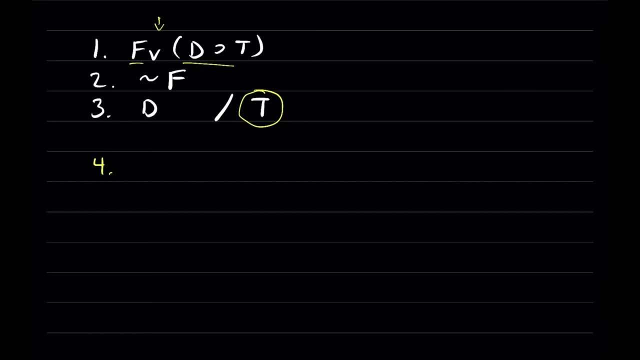 All right, this is a disjunct, either F or something else, but we know F is false. That's a disjunctive syllogism. It looks like this: P or Q, not P, therefore Q, And here Q. 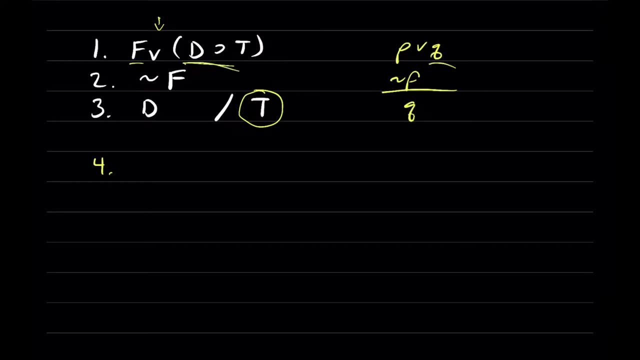 would be: D implies T. It's a complex statement But you can see this matches the pattern for disjunctive syllogism DS. So on line number four, we know that if we have the negation of that first disjunct, the second disjunct has to be true. And the second disjunct in this case is: 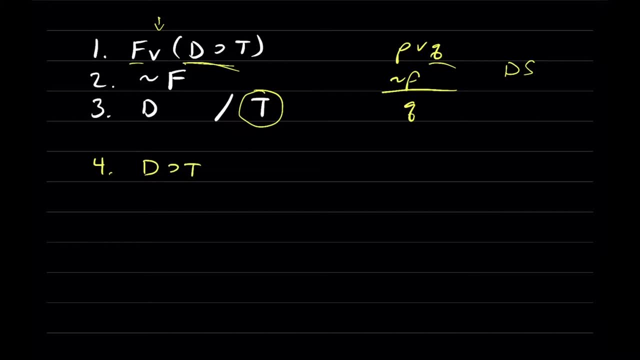 this statement, in parentheses, D implies T. Now, when you're doing a proof, you have to cite what premises you concluded that new line from and the rule that you used to deduce it. So in this case this new statement D implies T came from line one and line two using the rule disjunctive. 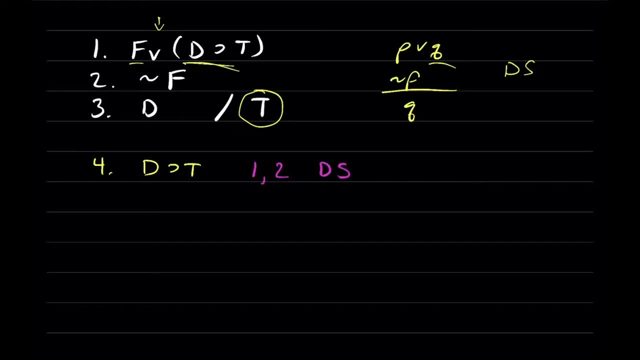 syllogism, DS And again, just to make it really clear, premise number one tells us either F is the case or D implies T. Line number two tells us F is false. So we know that D implies T has to be true. That's what. 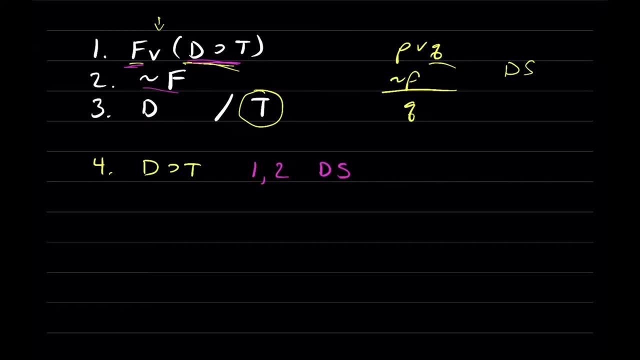 disjunctive syllogism does. All right, let's keep going here. Well, our new line, line number four, says: if D, then T or D implies T, And line number three tells us that D is actually true From those. 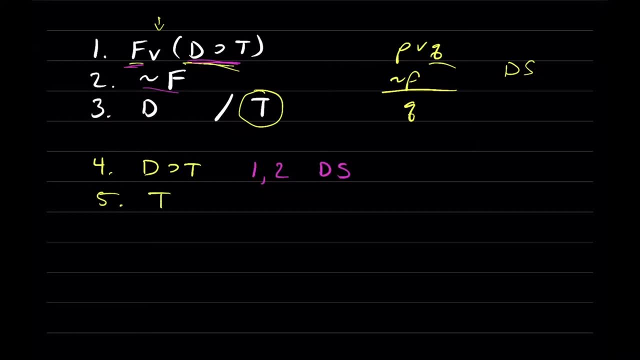 two statements we can conclude that T has to be true. And why is that? Well, it comes from line three and line four. According to the rule, modus ponens MP- And if you remember, modus ponens was P- implies Q. 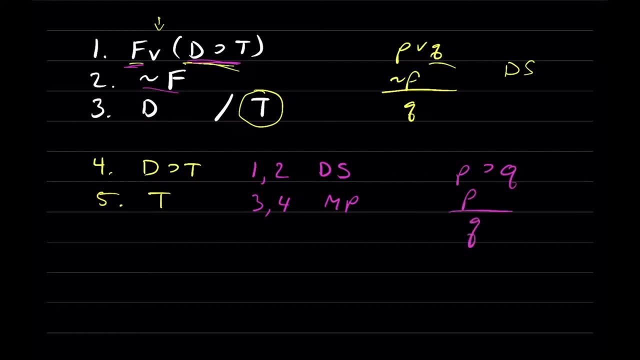 P, therefore Q, And that's what we have going on here. We have: if D, then T. D is true. therefore, T has to be true And we're done Once we've reached the conclusion on its own line. we've shown that the argument has to be valid, that the conclusion T. 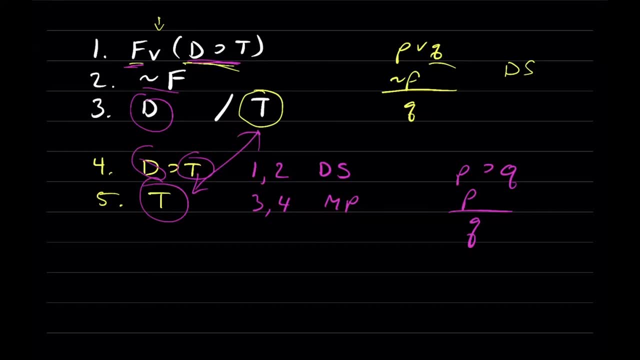 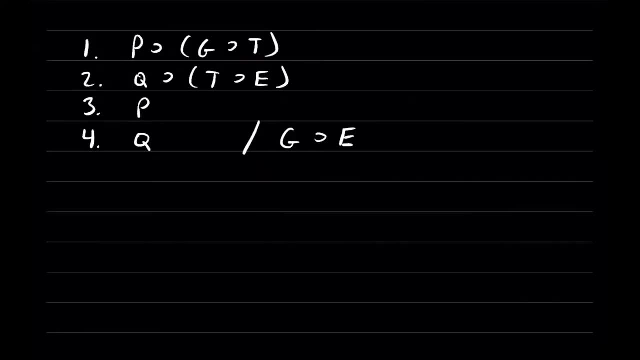 necessarily follows from the premises that are given. Okay, let's go on. Let's do another example. In this argument on the screen, we've got four premises that are given to us. P implies that, G implies T. And again, the main operator here is this horseshoe. 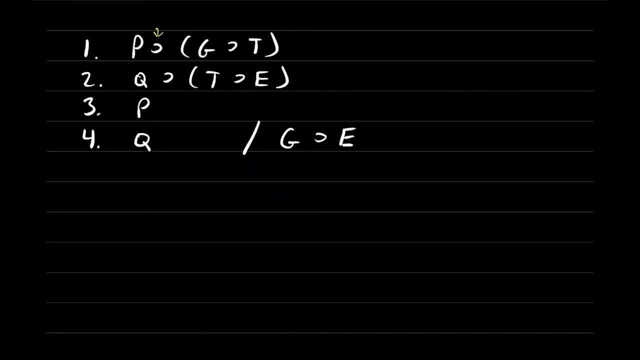 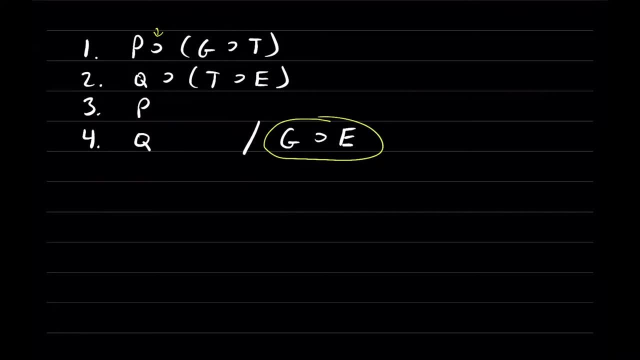 G implies E on it's own line will have shown that this argument is valid. Let's go ahead and dive in. We're going to add a new line, line number five, And there are a couple of starting places here. Line one tells us that, if P is true, something 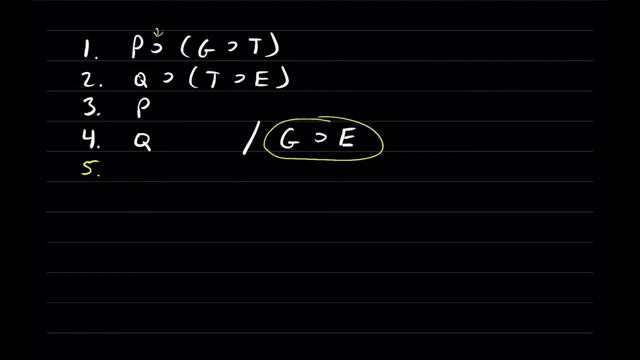 follows from that. And line two tells us that if Q is true, something follows from that. And lines three and four tell us P and Q actually true. so we could start with either one of those two conditionals. Let's just start with the first one. If P is true, then we know that G implies 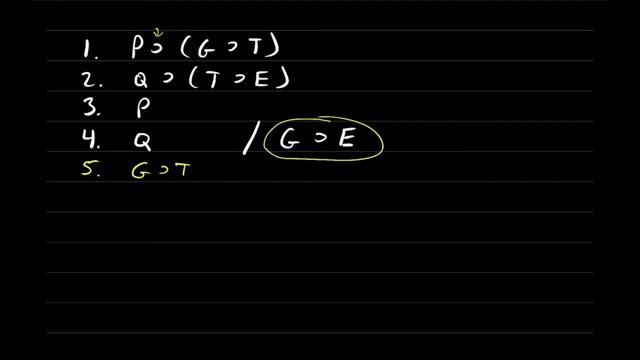 T. That's because line one tells us if P is true, then we get that conditional inside parentheses. Line three tells us that P is actually true And that follows from line one and line number three by modus ponens. And again just to be really clear here, modus ponens is: if P, then Q. 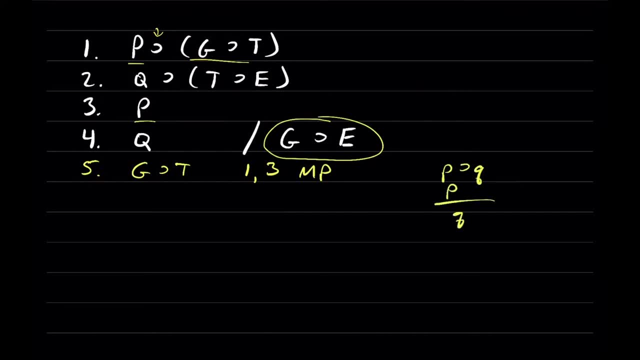 P, therefore Q: Okay, Let's keep going. Line two now tells us- I should say, this is what's a little tricky about doing proof: There's nothing in the proof that tells you what exactly to do next. You have to start looking for patterns, applying the rules that you notice, hoping that. 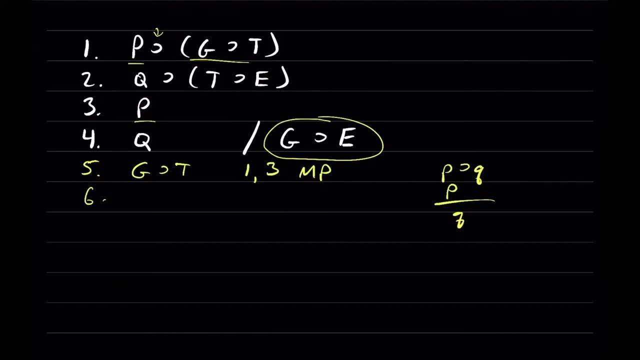 it's going to lead to that conclusion. That's why proofs are not a decision method. If you don't see what to do next, that doesn't mean that the argument's invalid. It just you didn't see what to do next. So this is not a mechanical plug and chug means of demonstrating. 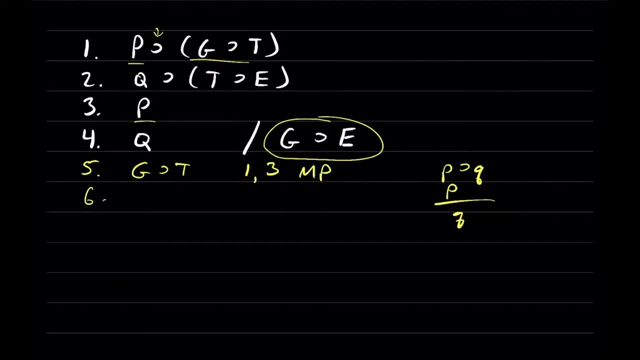 that any given argument is valid. It takes a little bit of intuition and a little bit of human pattern recognition to demonstrate that any given argument is valid, to see what rule to apply next. So what I noticed next is that line two right here tells us that if Q is true, this expression: 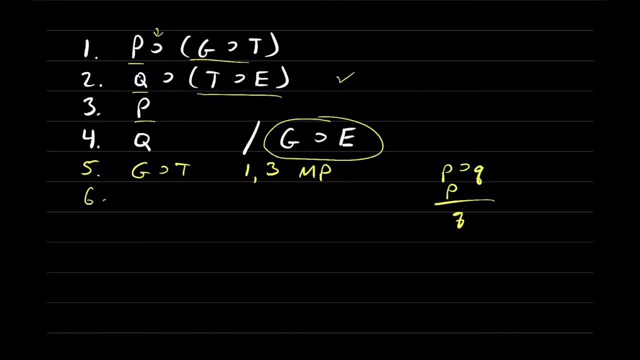 in parentheses has to be true. T implies E, But line four down here tells us that Q is actually true. From those two things we can conclude that T implies E, And that follows from line number two and line number four by the same rule: modus ponens: if P, then Q, P therefore Q. 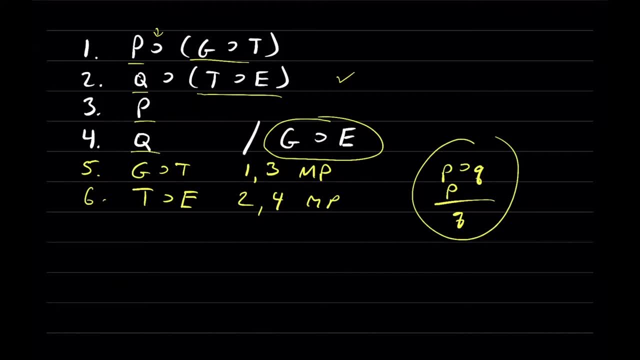 We're not done yet. We don't have G implies E on its own line, So let's add a new line and see what we can find. Well, line number five tells us that if G is true, we can get T from that. 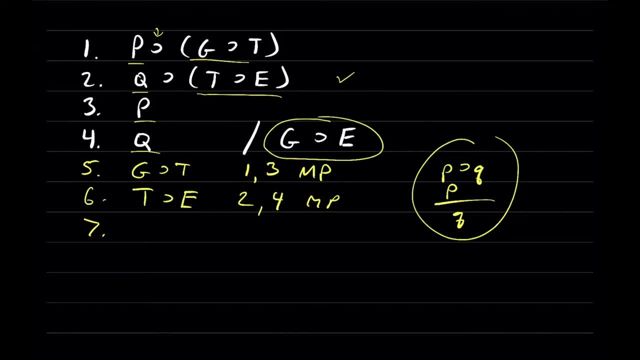 But six tells us that if T is true, we can get E from that, right. If T, then E. That looks an awful lot like a hypothetical syllogism. G implies T, but T implies E, And you can conclude from that that G implies E. And if you remember, I'm going to write it way up. 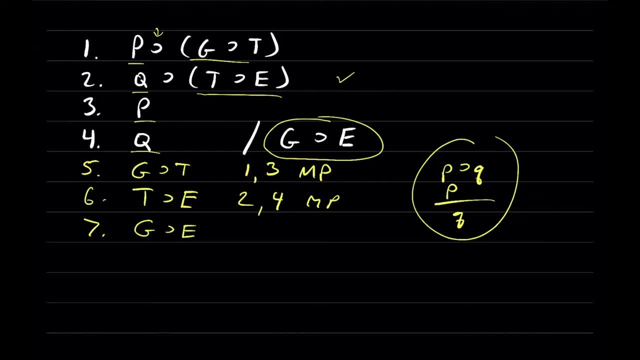 here. This is according to the rule hypothetical syllogism. If P implies Q, but Q in turn implies something else, let's call it R. then we can get P implies R from that. That's exactly what we're going to do next. So let's add a new line and see what we can find. 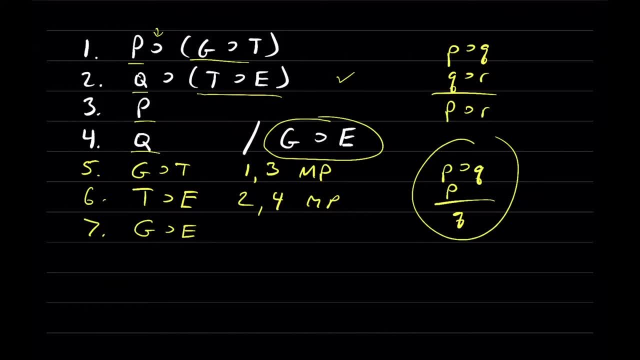 So what we have going on here, G implies T, that's our P and our Q. T implies E, that's our Q and our R. So G implies E, And this would follow from line five and line six by hypothetical syllogism. 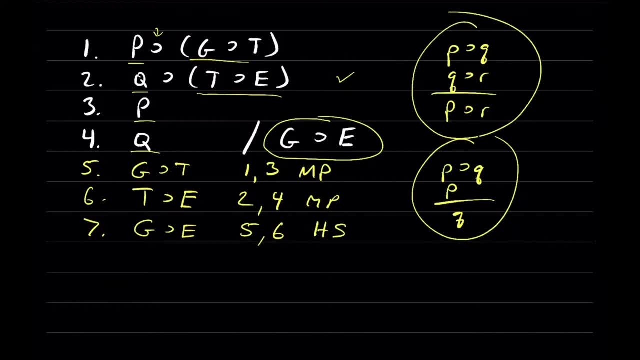 HS this rule right here. So you can see this is a lot more elegant than doing a proof And in fact, if you look at this argument, we have P G T E, P G T E and Q: five lines. That means we: 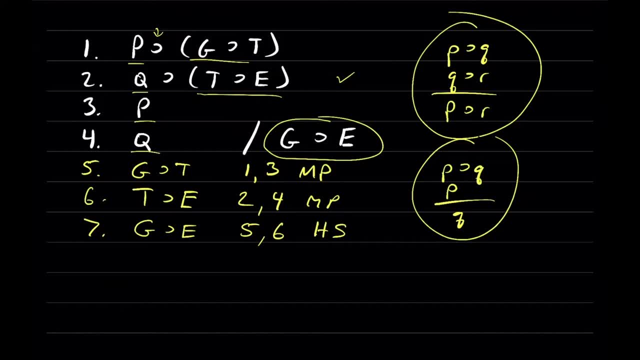 would have two to the fifth. So you can see, this is a vastly more elegant way of showing that arguments are valid. The downside is it does take a little bit of intuition and a little bit of pattern recognition to find these argument patterns in these compound statements that make up the argument. Okay, let's keep going. 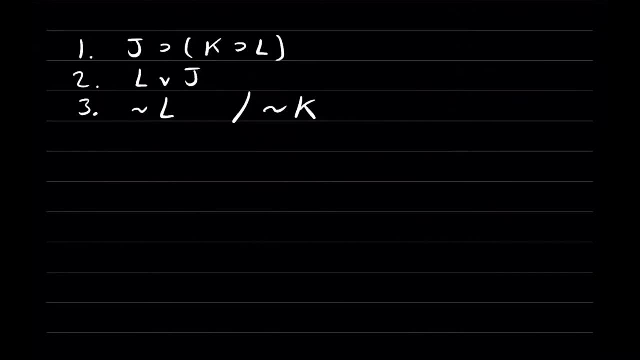 I want to do a lot of examples for you. The next argument I've got for us here is: it's got three premises. J implies that K implies L. So if J, then this expression in parentheses, K, implies L. The second premise says either L or J. it's a disjunction. And line number three says: 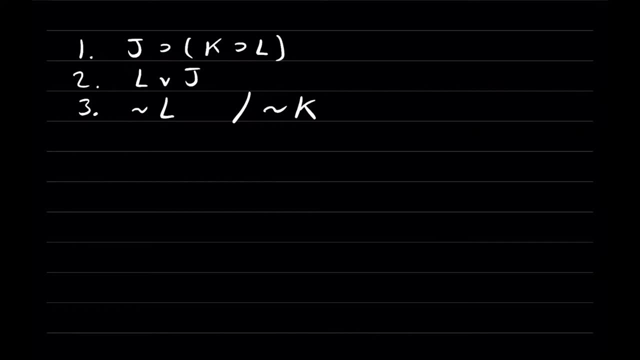 not L, And the conclusion that we're trying to show follows from these premises is not K. So when we get not K on its own line, we will have shown that this argument is a valid argument. Let's dive in. We're going to add a new line, line four. 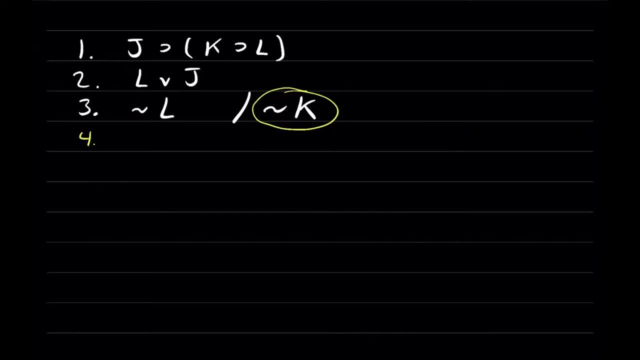 Right off the bat I noticed that lines two and three look like a disjunctive syllogism. A disjunctive syllogism is either P or Q, not P, therefore Q Right Over here on the left. 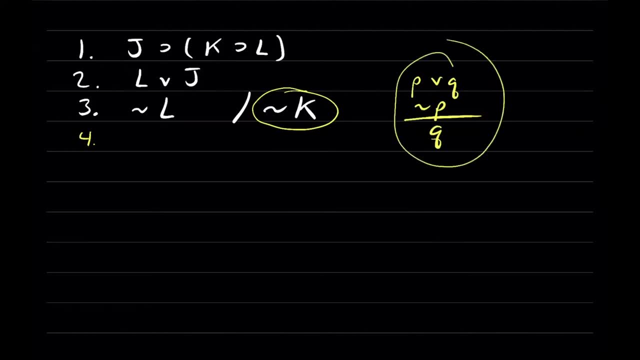 we've got L or J and not L, Same exact pattern as what you see here in the argument form. So from that we can conclude that J is true. And again, I just want to make sure this reasoning is really clear. This is super easy reasoning right. Line number two tells us either L or J is true. 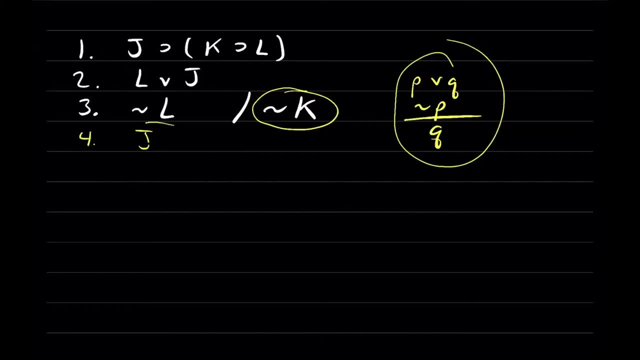 Well, if L or J is true, then it's true. So if L or J is true, then it's true, And if L or J is true, if one of them is false, not L- we know that J has to be true. That's what a disjunctive syllogism. 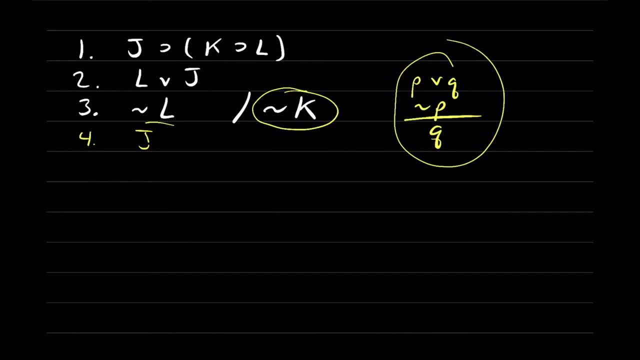 is. So this would follow. I'm going to change color here to make this easy to see. This would follow from lines two and three by disjunctive syllogism: D S. Okay, Once we have J, notice that line number one says: if J is true. 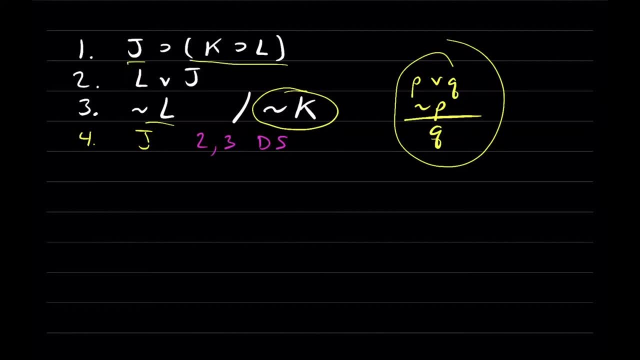 then something else has to be true. This expression, inside parentheses, And line number four, says: if J is true, then something else has to be true. This expression, line number four, happily tells us that J is true. So on line five we can conclude this consequent. 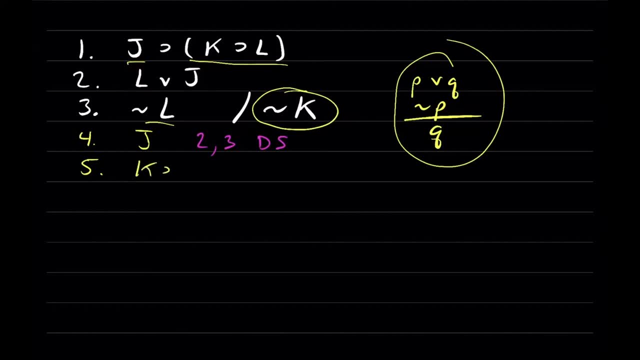 of this conditional in line one: if K, then L. And again, just to make it really clear, line number one says: if J is the case, then all of this in parentheses is the case. Four says J is actually true. So we know from that that K implies L And that's going to follow. 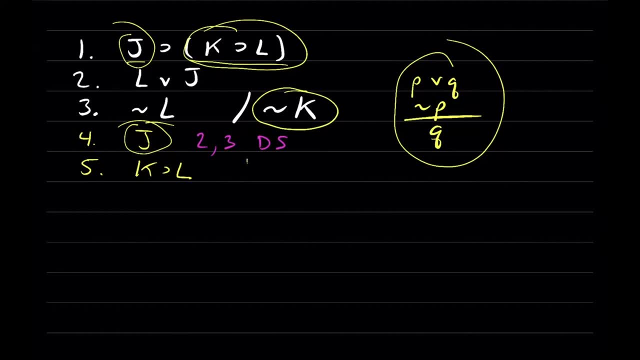 now from line. let me change color again here. That's going to follow from line one and line four by modus ponens, the rule that we looked at a couple of arguments ago. At a certain point you'll have to commit these argument forms to memory. It just takes practice. 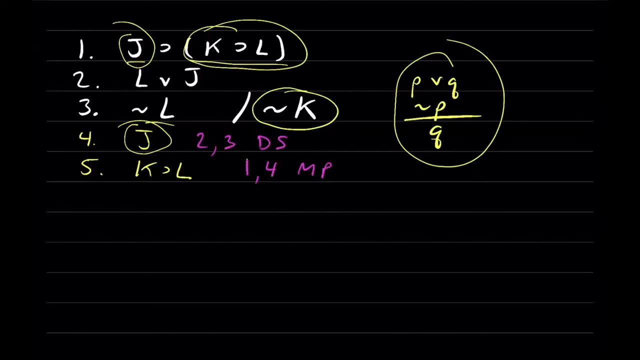 and practice, and practice. So while you're doing the proofs that make up the exercises for your homework, just have the book open and have that list of rules right in front of you So you can see the argument patterns. I don't expect you to have all of these memorized right off the bat. 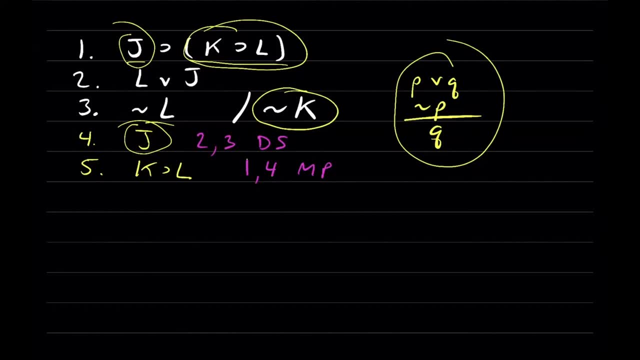 have them there with you. It'll take practice and practice and practice, though, for you to be able to and instinctively notice the patterns that make up these argument forms inside the argument you're given. That's why you have to do so many arguments for homework, for practice. Again, logic is very. 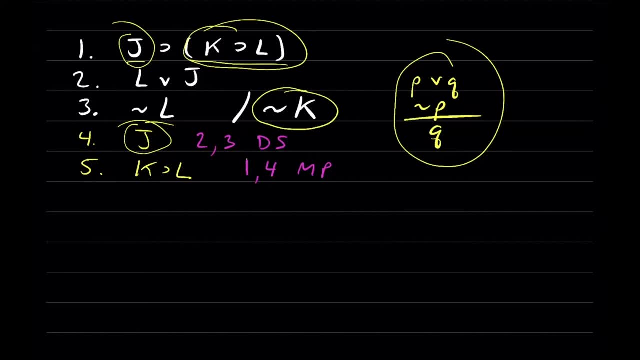 practice-based. Unless you kind of train your mind to recognize these patterns, it's going to be very difficult to plug and chug through all these proofs. Okay, let's keep going. We're going to add a new line, line six, and let's see what we can conclude. Well, in line five we have a new. 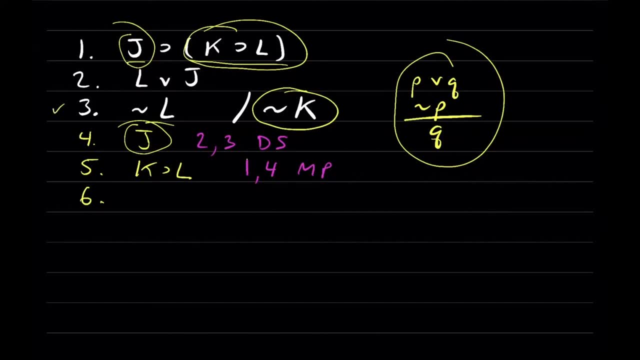 conditional K implies L, But line three way up here tells us that L is false And that looks like the argument form for modus tollens. and that is: P implies Q. If Q is false, that means P has to be false, And that's. 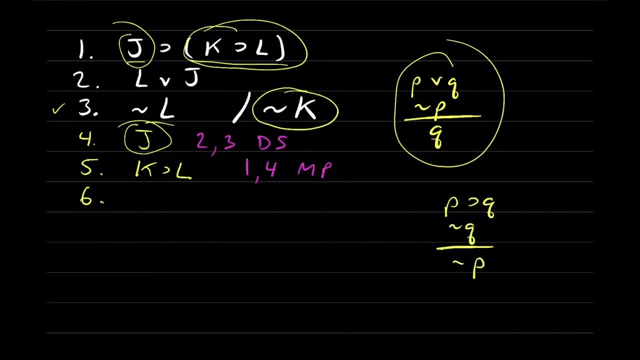 what we have going on here. We have K implies L right here. We know that L is false right here in line three. From that we can conclude that K is false, not K, And that follows from line three, line three and line four. 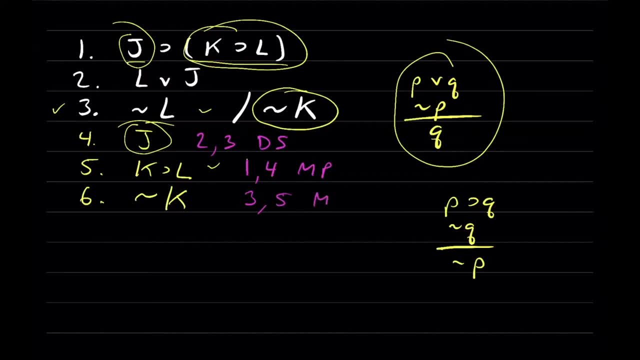 Line five by modus tollens, M, T And again. once you get that conclusion on its own line, you're done with the proof. We've got not K on its own line. Every line new line that we added is a valid argument step, valid inference step. So that conclusion has to follow from those. 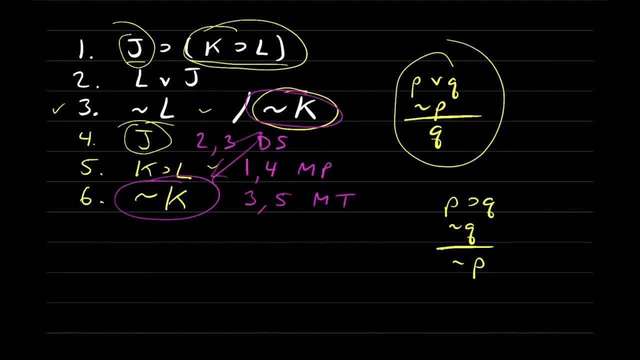 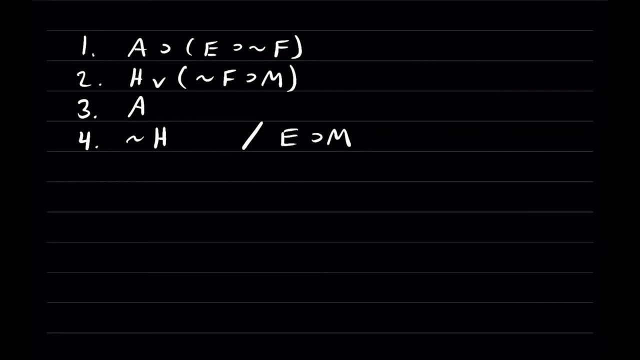 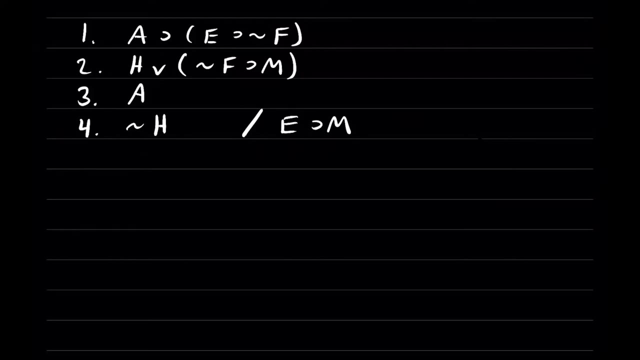 premises Again. second: you get that conclusion on its own line. you're done Pretty straightforward. Let's do a slightly more complex proof. So in this proof you're given four premises. If A, then E implies not F. Kind of a lengthy first. 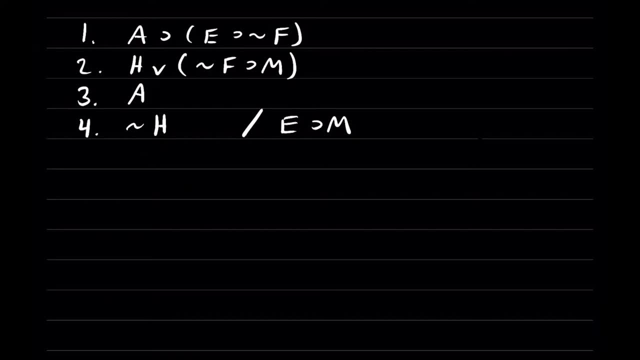 premise. Line number two says either H- it's a disjunction- either H or not. F implies M. Three just says A is true and four says H. H is false, not H. So we're going to start out by adding. 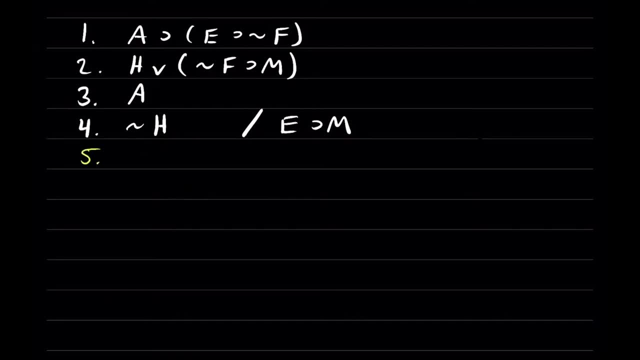 a new line five and we'll see what we can deduce from this. I think the easiest thing to recognize here is that line one is a continuous line, Line two is a continuous line, Line three is a continuous line, And in line three you've got the antecedent of that conditional A. So again, just to make this, 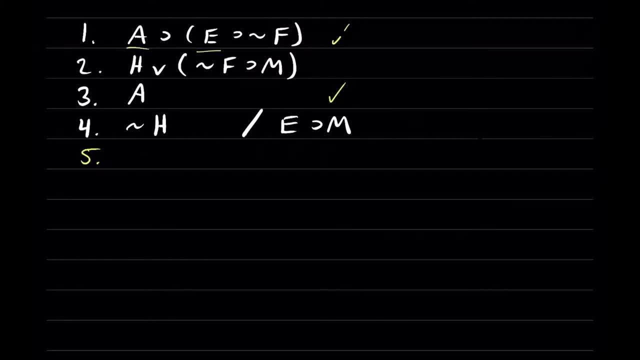 really clear. line one says: if A is true, then this entire expression in parentheses has to be true. And line three tells us A is actually true. That means the consequent of that conditional inside parentheses has to be true. So we're on its own line. now We're going to get. E implies not F. 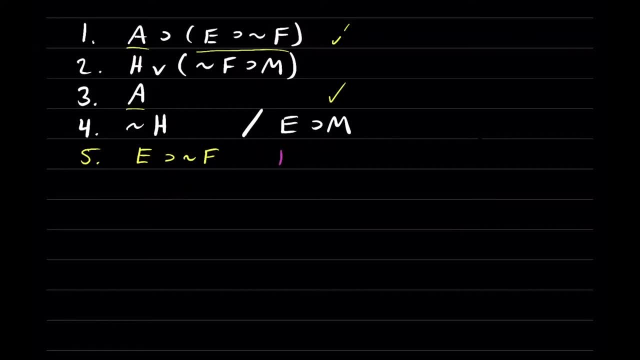 from line one and line three by modus ponens. Okay, And again, just to be really clear, modus ponens: if P implies Q, P, therefore Q. Okay, Add a new line, line six. The next thing I notice is that line number two is a disjunction. 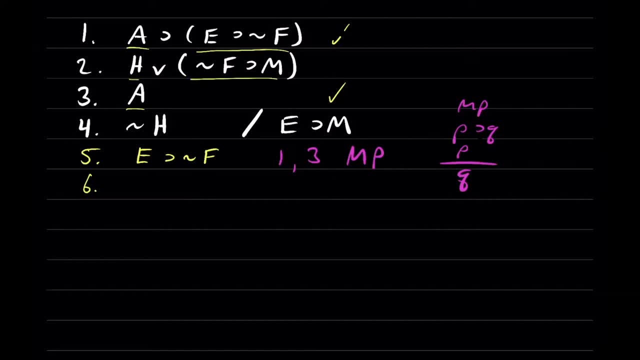 It says either H is true or this expression in parentheses has to be true. But line number four right here tells us that line four is a disjunction, So we're going to get E implies, not F, H is false. That means that this expression in parentheses has to be true, And that to me, 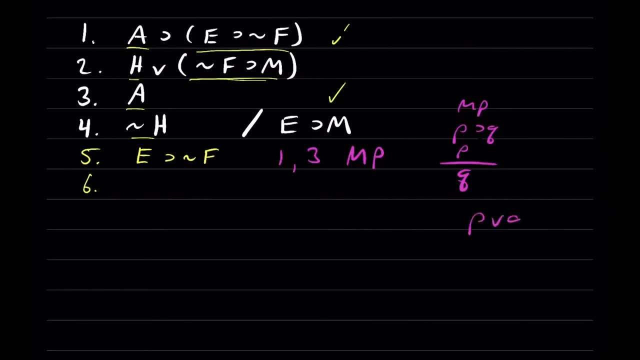 looks like the form for disjunctive syllogism: P or Q, not P therefore Q. So on line six we're going to get this expression inside parentheses. not F implies M. According to what rule? now, Let's see, It's going to come from line two and line four by this rule. 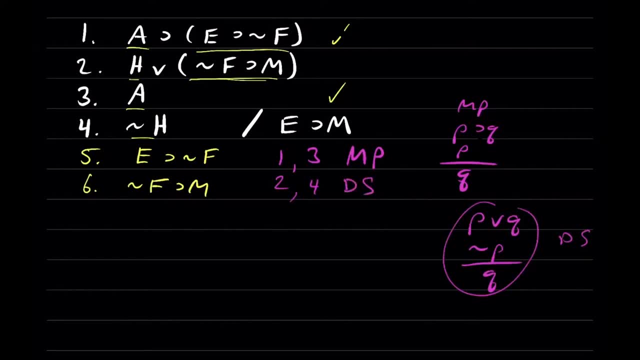 here. disjunctive syllogism, DS. Okay, Let's see what else we've got. Okay, What I noticed next is that in line five and line six you've got two conditionals where the same term, not F, is the antecedent of one and the consequent of the other. 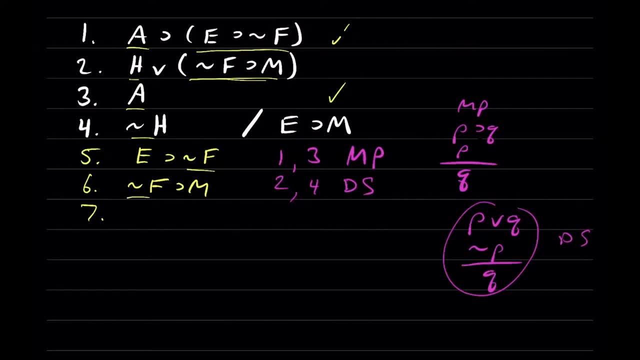 And if you kind of just naturally speak through the reasoning here, you should be able to see what follows from this. Line five is the antecedent of one and the consequent of the other. Line five says E implies not F. Line six says that not F in turn implies M From that. 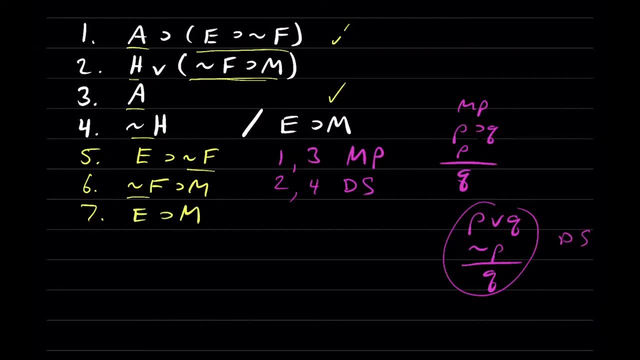 you can conclude that E implies M. Again, just talk through the reasoning. If E, then not F. line six says: but if not F is the case, then M has to be true. So you know that if E is true, you have to get M. If E, then M. And that's going to follow from line five and line six by: 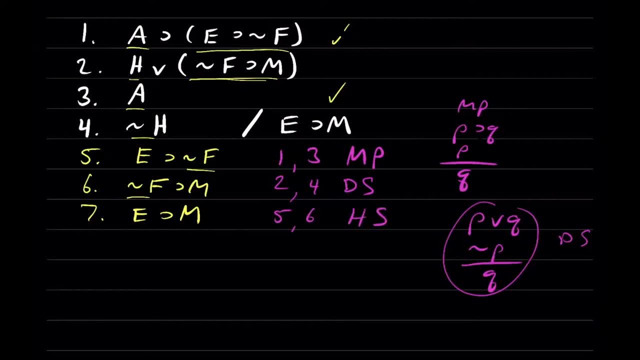 hypothetical syllogism, HS. And just as a reminder, hypothetical syllogism is this: If P then Q, If Q then R. Therefore, if P then R, HS, Hypothetical syllogism. Okay, From this point on, I'm not going to keep drawing out each of. 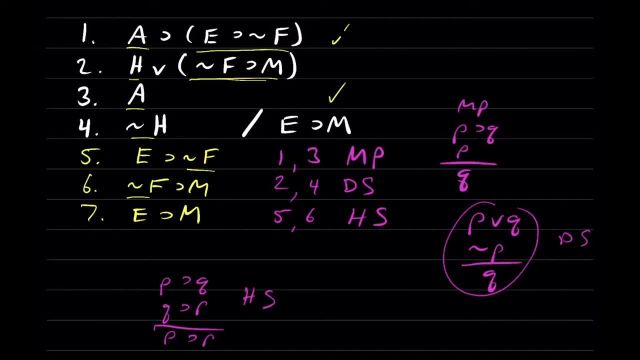 these rules. You should be able to follow along with the rules inside your textbook and we should be able to speed through the rest of these arguments. If you're having trouble committing these arguments to memory, talk through the reasoning behind them, You know, pronounce them. 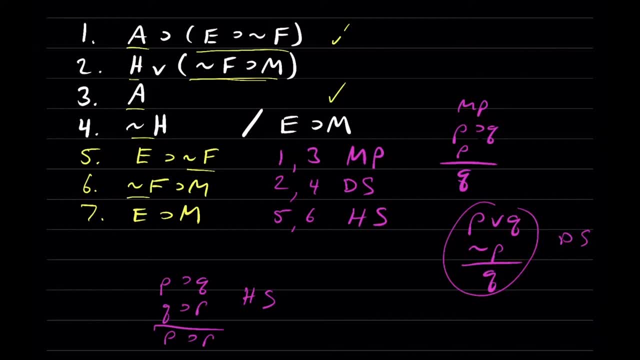 like I'm doing here. If P, then Q, But P is true. Therefore, you have to get M, And that's going to follow from line five. So you know, pronounce them like I'm doing here. Therefore, you have to get. 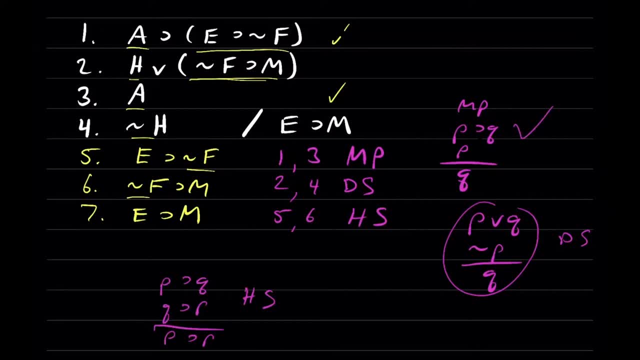 M, And that's going to follow from line six. So you know, pronounce them like I'm doing here. That's modus ponens right here For disjunctive syllogism. the first premise says either P is true or Q is true, But the second premise says P is false. You know from that that Q has to be true. 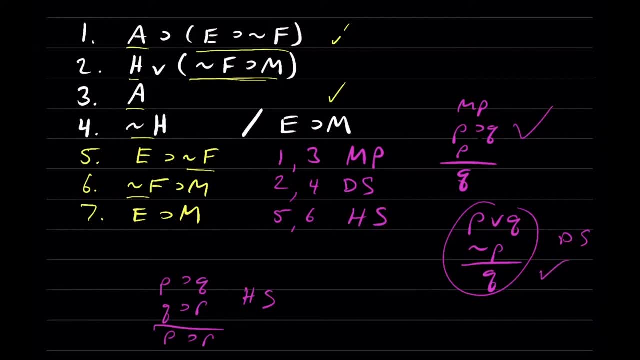 That's what disjunctive syllogism is. So if you try to just brute force memorize these without really paying attention to what they mean, you're really setting yourself up for a challenge. But if you talk through the reasoning, I hope you can make these rules intuitive and you can see. 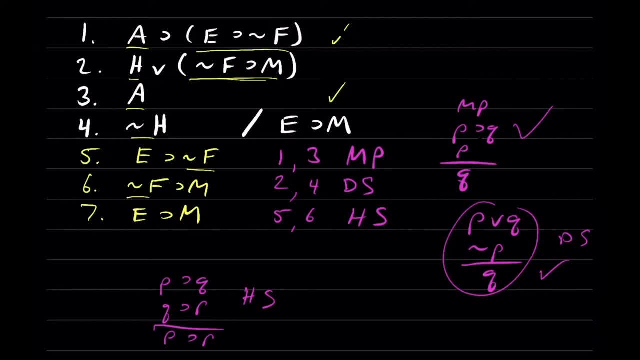 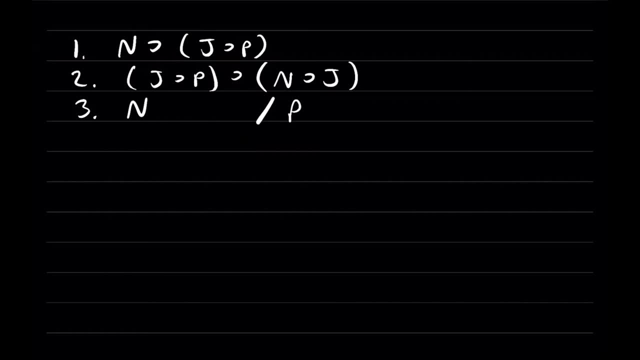 the reasoning behind them, See why they're valid and why they work. Okay, Let's do a couple more examples. examples: Okay, in this argument we have three premises. Line one says: if n is the case, then j implies p. Line two says: if j implies p, in other words, if all this in parentheses, then n implies. 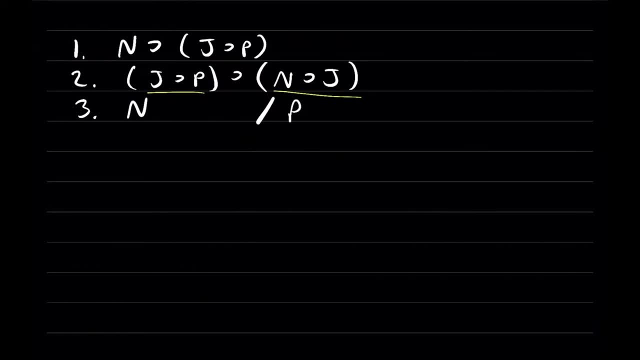 j, all that in parentheses. And line three says n is true, just n on its own line, And we're trying to show that p is true. So the second: we get p on its own line using a series of valid deduction. 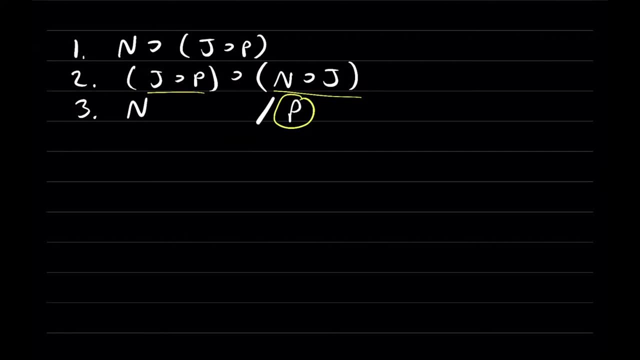 rules, valid deduction steps will have shown that this argument is valid. So we're going to add a new line, line four, and see what we can deduce Right off the bat. I noticed that line three is the antecedent of the conditional in line one. Line one says: if n is true, then j implies p And we 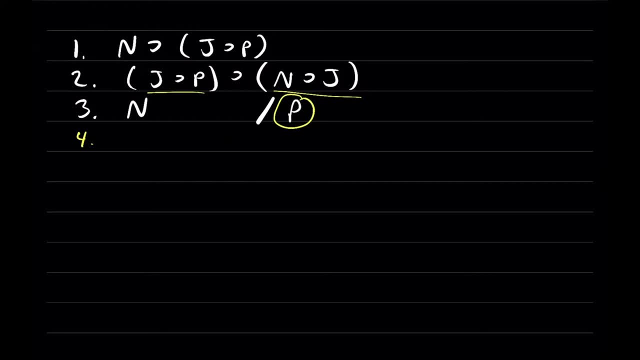 know that n is true from line three. So from there we can conclude that j implies p, And that's going to follow from line one and line three by modus poni. Okay, Notice now. now this is where things start to get a little tricky, And I'm just going to 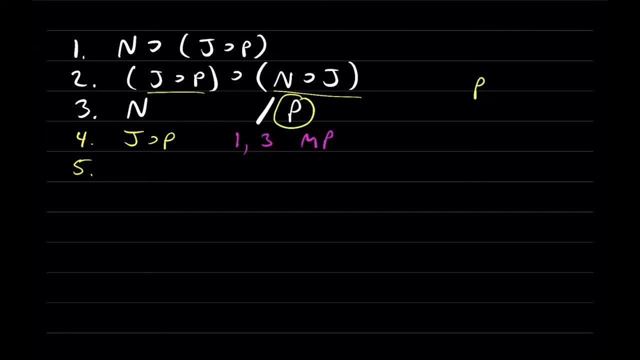 write it out here. So I'm going to refresh your memory on modus poni. If p then q, p therefore q. This is modus poni. Hopefully it's already review and you've already got that one down. 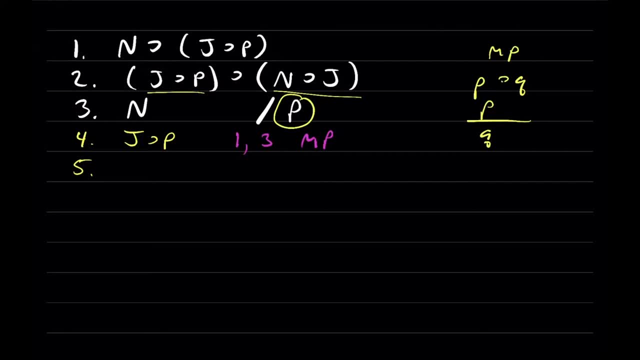 the easiest one of the bunch. But here in line two and four, we have an argument that matches that pattern. All of this j implies p would be p in this argument form, right here. And all of this in parentheses right here would be q in this argument form, right here. And line four: 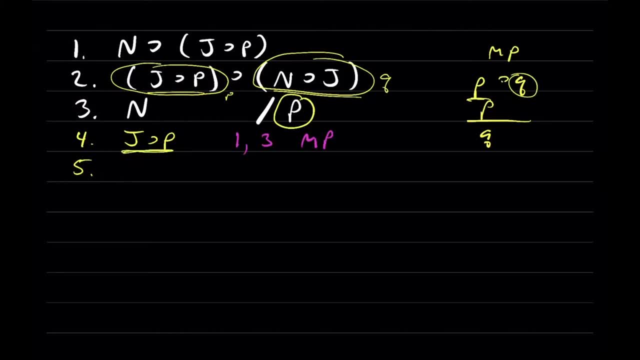 is the antecedent of that conditional. j implies p. Again, I'm just going to put it in a little subscript here. This is p right here in the argument form. So that says that we know that the consequent of this conditional in line two has to be q. So we're going to add that to the 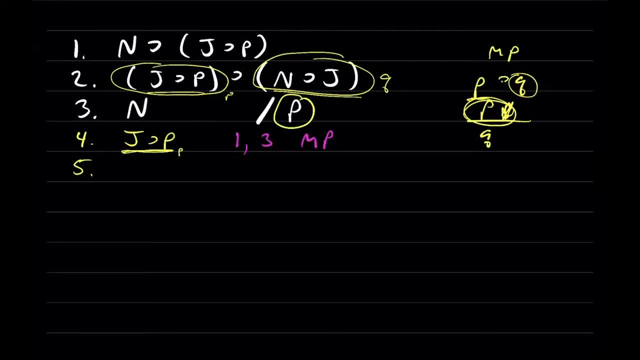 be true, And I think you can see this and I'm just going to draw circles around it. Even though this is going to make the argument a little ugly, I want to draw explicit attention to it. Line two says: if all of this- that I've circled here in yellow, that I'm circling right now- is true, 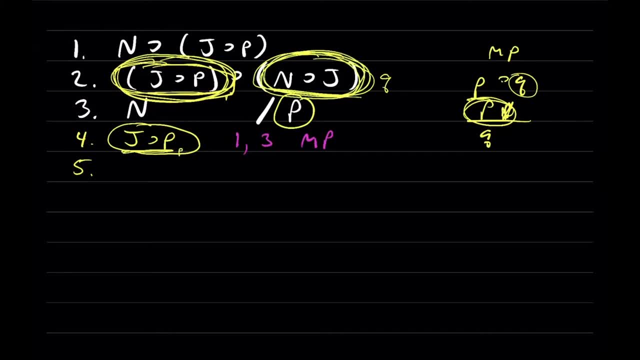 then all of this has to be true. The second expression in parentheses, N, implies J. Line four tells us that first expression is actually true: J implies P. So we know from that that N implies J, the second expression in parentheses, And that is the form for modus ponens. 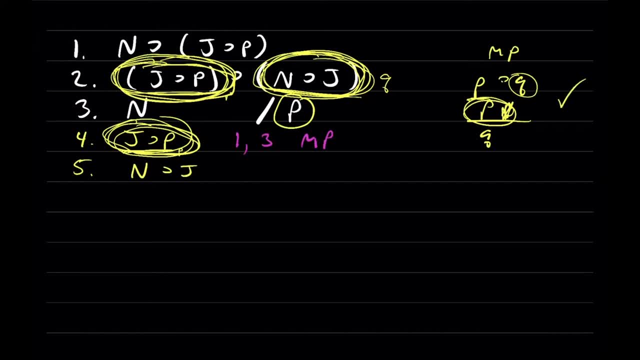 But here P and Q don't stand for simple statements, just simple capital letters. They stand for complex expressions in parentheses, And you have to be able to recognize that in order to be able to do proofs effectively. Okay, so every time you get a new line, you have to cite the lines that it 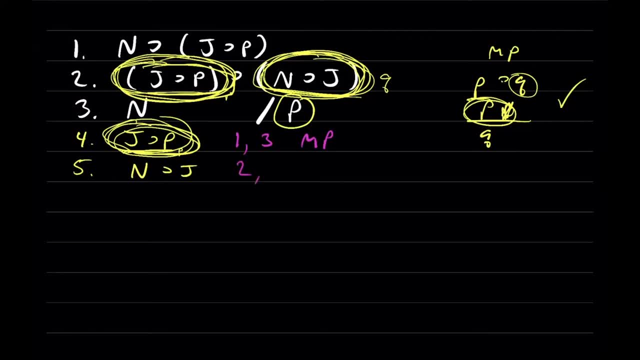 comes from and the rule that you use. So this came from line two and line four by modus ponens: If P, then Q, P, therefore Q. Okay, Well, there are a couple of things we can do here. What I noticed next is that in lines four and five we have two conditionals and the antecedent. 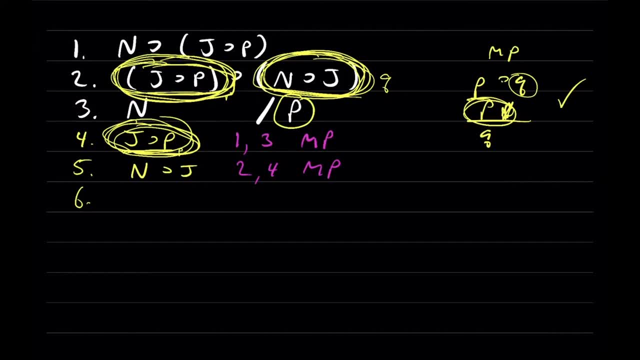 of one conditional is the consequent of the other. In line five we have N implies J, but line four tells us that J implies P implies P, And that is the form for a hypothetical syllogism. So from that we can get N implies P. 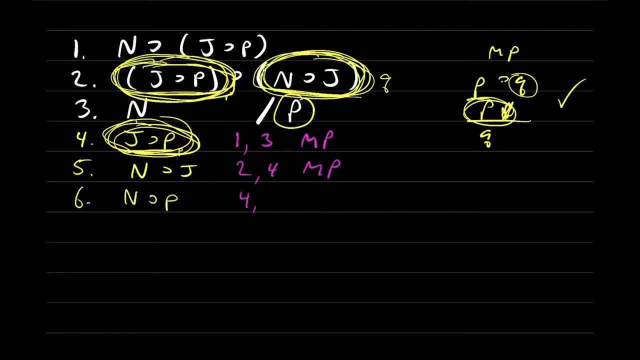 And that would follow from lines four and five by hypothetical syllogism HS. Okay, we're almost done here. This new conditional that we got on line six, N implies P is a conditional. If N, then P. But way up here in line three we already knew that N was true. And from those two lines 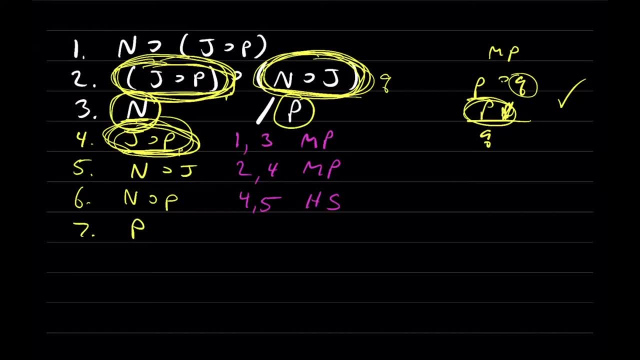 it follows that P has to be true, right? If N, then P, and we know N is true. P has to be true, And that would follow from line three and line six by modus ponens, And once we get P on its own line, we're done Right here. Okay, so we've shown that that. 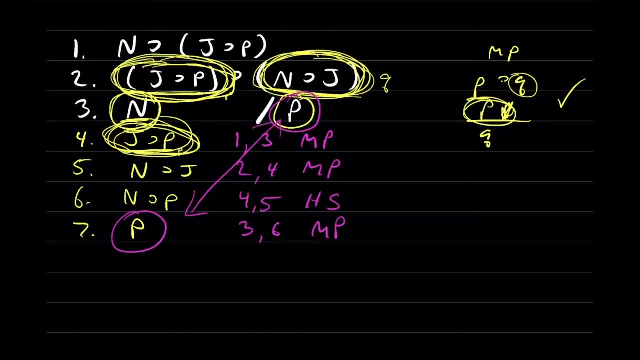 argument is valid and it only took four additional lines. So, as you can see, proofs are a pretty elegant way of showing that arguments are valid. Okay, I've been marking these up a lot to demonstrate the patterns that I'm using to help you identify visually the patterns inside the argument. I'm going to try to be a little. 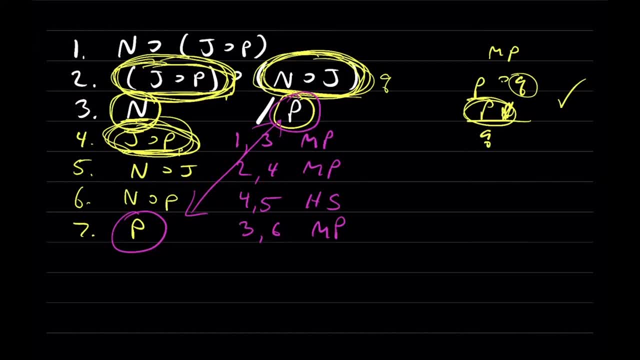 cleaner from here on out and produce fairly polished finished proofs. And if you need a reminder on any of the rules you know, pause the video, go find the argument forms that I'm citing inside the textbook, look at the argument that I'm doing on the screen and 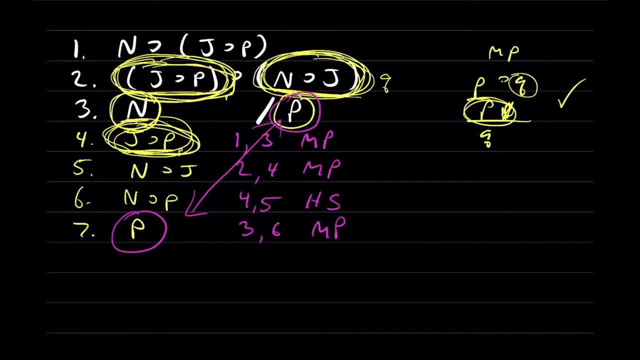 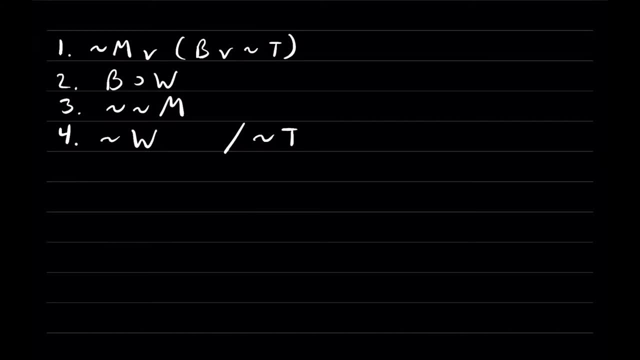 follow along and see if you can identify that pattern every step of the way. Okay, so this argument is looking a little scarier, but it's pretty straightforward still. We've got four premises. Line number one says: either M is false or this expression in parentheses has to be true B or not T. 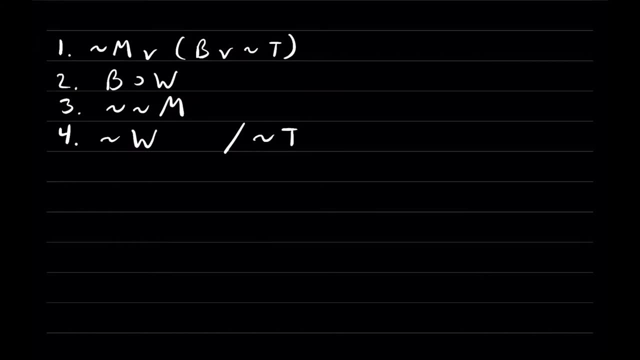 Line number two says B implies W. Line number three is not, not M. Now, this is going to look a little strange if you haven't seen this, but you can have a negation of a negation. Of course, not, not M is just M. line number three is not not M. Now, this is going to look a little strange if you haven't seen this, but you can have a negation of a negation. Of course not. not M is just M. This is a double negation. 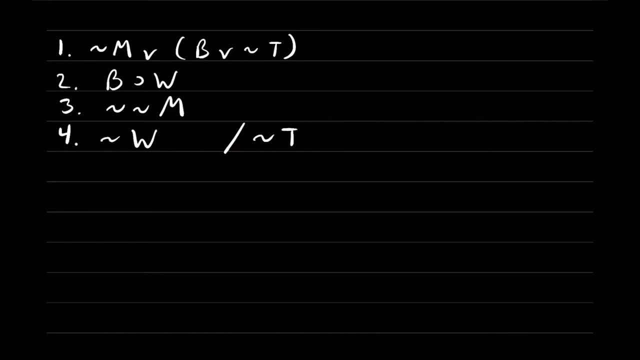 Later in the course, there's going to be a rule that lets you cancel out double negations like this, but you don't have that rule yet. The way to think of this is that this is a negation of, not M, right here. 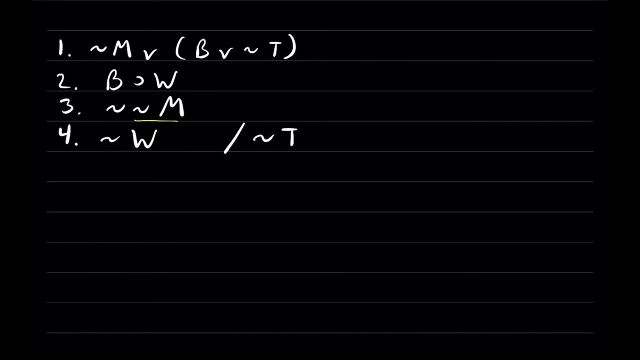 So not M on its own is obviously the negation of M, Not not M would be the negation of not M. So be really careful with these double negations. when you see an example like that, You can't just eliminate them yet You don't have that rule yet. There is a rule that's coming, but the textbook doesn't introduce that to you. 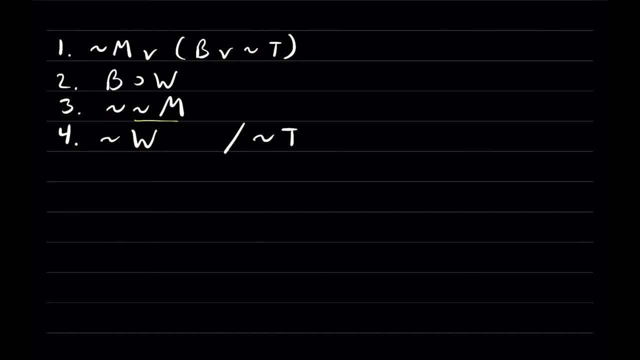 Just yet. And line four says: not W- And we're trying to show this conclusion- not T. Let's dive in, Add a new line, line five. The first thing I notice is that line three, not not M, is the negation of this disjunct right here in the first premise. The first premise says: either not M or this expression in parentheses, this expression in parentheses B, or not T. 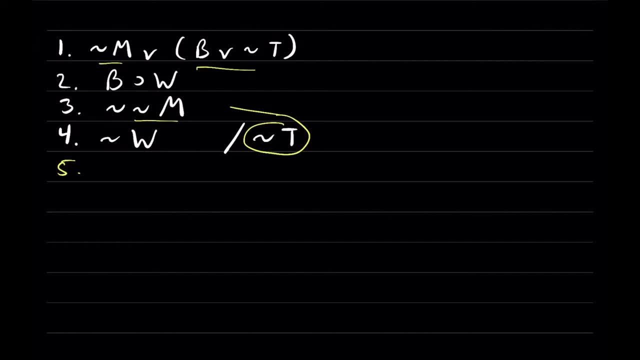 Three is not not M, So we know that first disjunct not M is false. That's what not not M, not not M means. So from that we can conclude B or not T, And that would follow from line one and line three by disjunctive syllogism, D S. 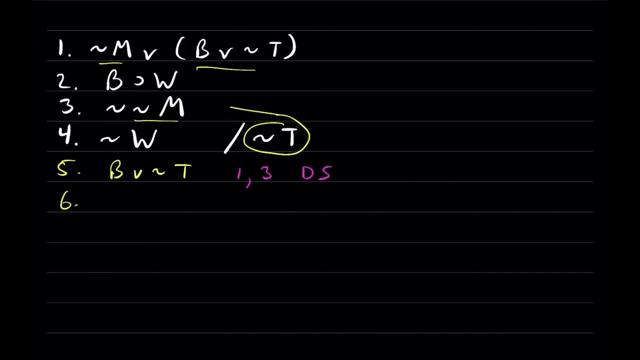 Okay, line six. The next thing I notice is that in line two we have a conditional: if B, then W or B implies W, And line number four tells us that that that consequent is W is false, not W. From those two statements you can conclude that the antecedent has to be false, not B, And that would follow from line two and line four by modus tollens. 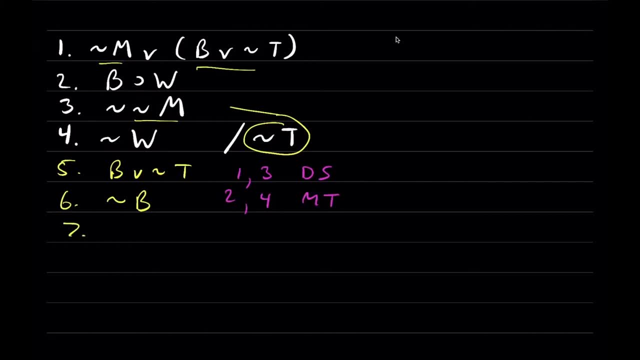 Okay, We're very close. We're very close to being done with this proof. Line five tells us that either B is true or not. T is the case. Line six tells us that B is false. So we know from that that not T has to be the case. right, This disjunctive, that disjunction in line five. 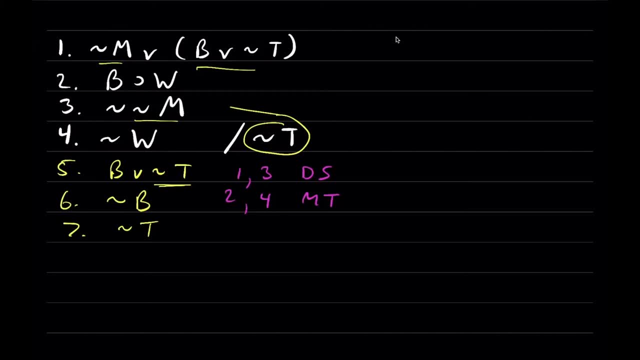 And that would follow from line five. excuse me, I'm trying to change colors here. line five and line six by disjunctive syllogism: D, S And we're done. We've got not T on its own line. 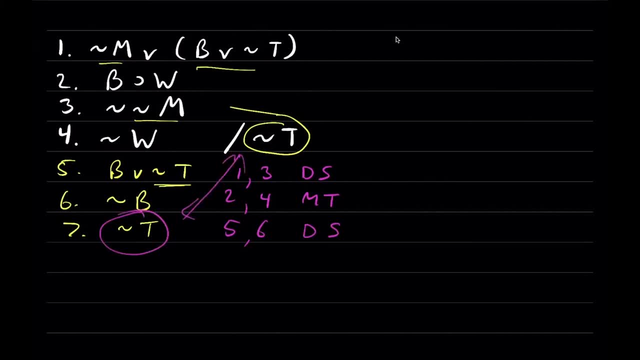 We've shown that that's true. We've shown that that conclusion follows from those premises. Only three lines it took. It was a fairly scary looking set of premises there But as you can see, it didn't take much to power through it and show that that conclusion follows. 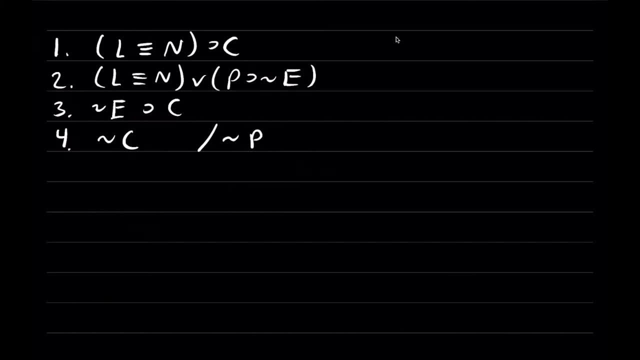 Okay. Okay, In this next argument we've got four premises. The first premise says: if L is equivalent to N, that's what that biconditional is. then C, Line two, says that either L is equivalent to N or C is equivalent to N. 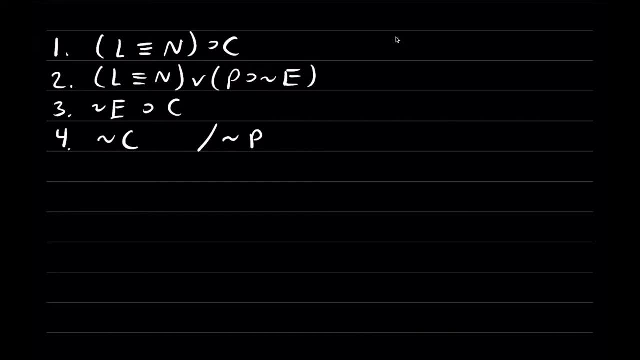 Line two says that either L is equivalent to N or C is equivalent to N, or C is equivalent to N, Or P implies not E. Line three tells us that not E implies C And line four tells us that C is false or not C, And we're trying to show this conclusion- not P. 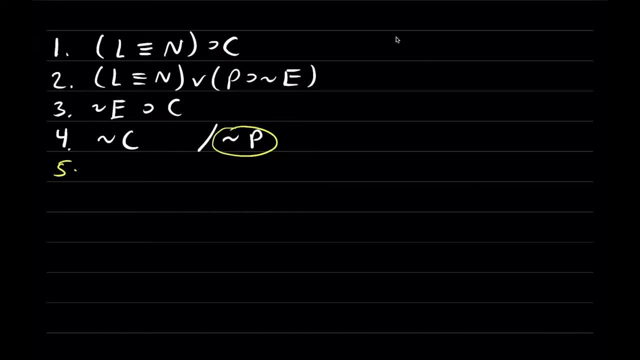 Let's dive in, Especially now. this isn't always true when you're doing proofs. but right now you want to look at the simple premises, Like there's not going to be much. there's not going to be anything you're able to do with the first two premises. 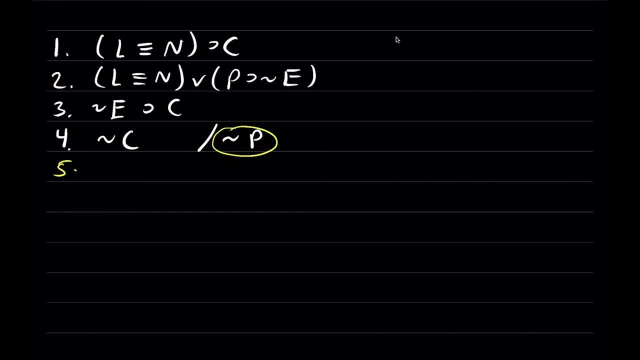 You know that kind of scary expression- L is equivalent to N- is kind of locked inside those parentheses. But you can do something with premises three and four right off the bat. So line three says if not E then C, And line four tells us that C is false. 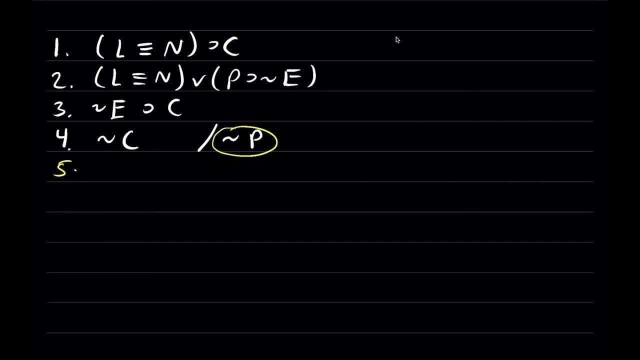 So that's going to match the pattern for modus tollens. We have the negation of the consequent here in the conditional, in line three. That means we know that the negation of the antecedent has to be the case, So that's going to be not, not E. 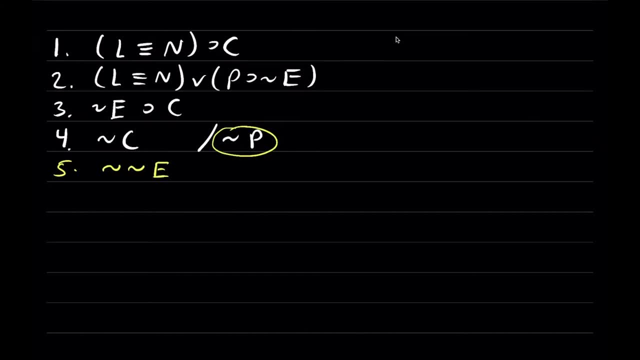 Here's our double negation. You've got to be really careful here. You can't just eliminate those right off the bat. You don't have a rule for that yet. So that's going to follow from line three and line four by modus tollens MT. 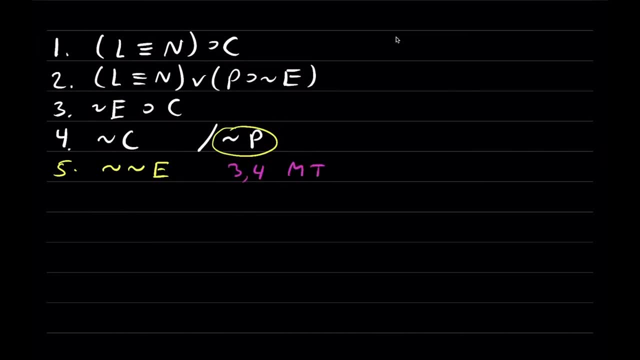 And again, if you're having trouble recognizing these patterns, you know, go back and watch the first couple of arguments I did, or pause the video and open up your textbook and follow along with the examples that are given of the definitions of the deduction rules. 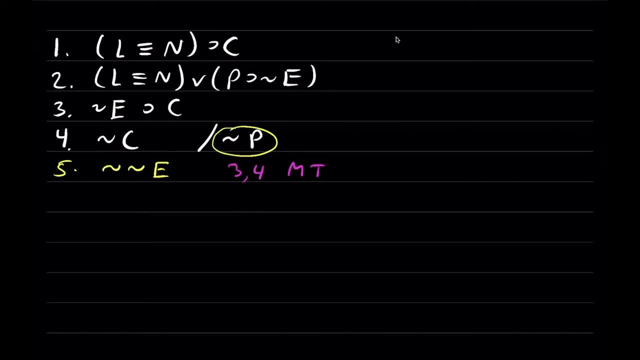 So you can see what I'm doing here And I think you can see, just to make it really clear, this is modus tollens is if P, then Q, we have the negation of the consequent not Q and we get not P as a result. 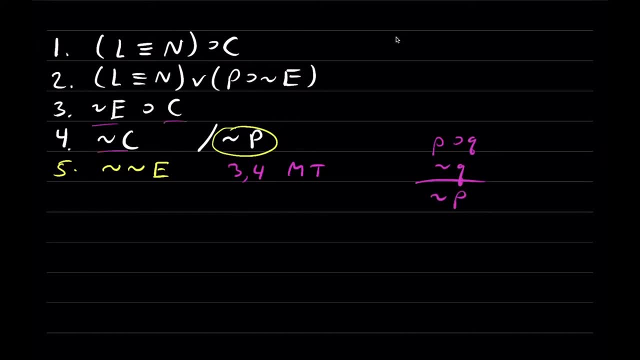 So here we've got our P and our Q. not Q, therefore not P. Okay, Line six. Well, the next thing I notice is that in line one we've got another conditional. If all of that in parentheses right here, then C: 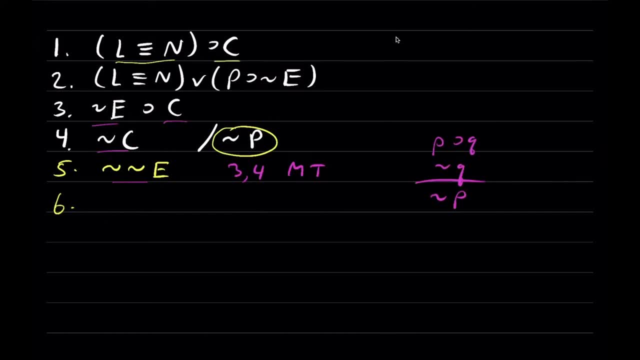 But we know C is false. Line four told us that, So from that we can get the negation of the antecedent of that conditional. The negation of L is equivalent to N And that's going to follow from line one and line four by modus tollens. 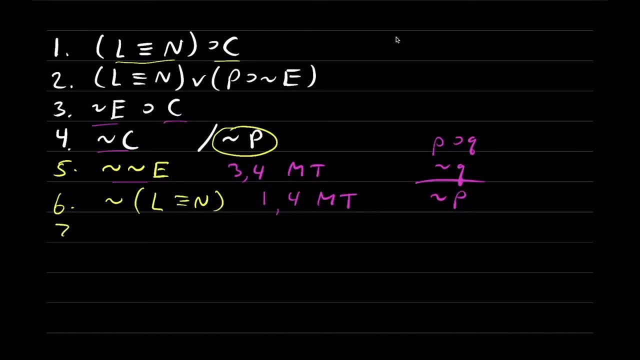 Okay. Well, line number two tells us that either L implies N or- I'm sorry, excuse me- either L is equivalent to N or P implies not E. But in line six we learned that that expression in parentheses L is equivalent to N is actually false, right. 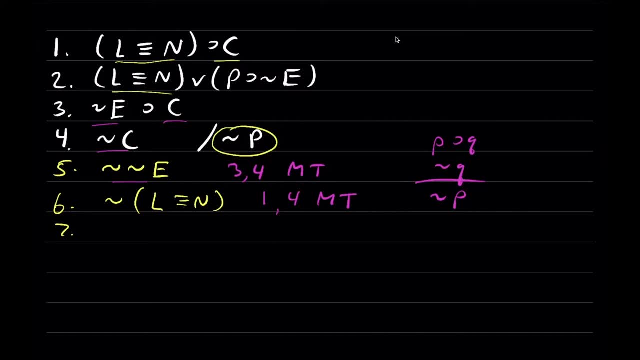 We have the negation of L is equivalent to N in line six. So from that we know that this other disjunction, this other expression in parentheses on the right side of that disjunction has to be true. So P implies not E. 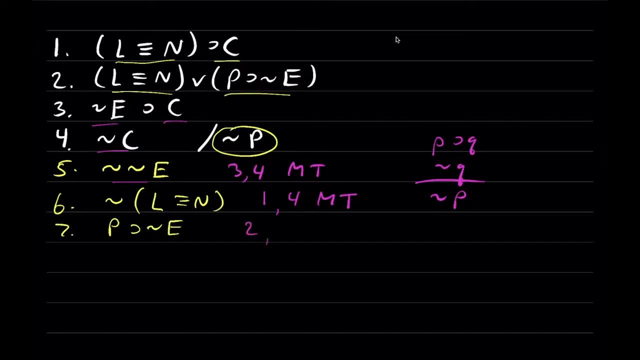 And that's going to follow from line two And line six. by disjunctive syllogism. And again just to make it really clear, line two says either L is equivalent to N. that's the expression in parentheses on the left. 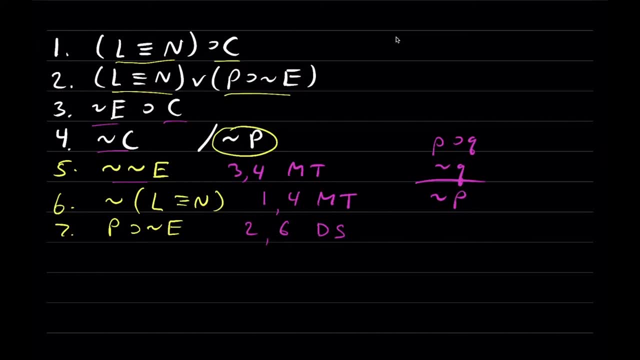 or P implies not E. that's the expression in parentheses on the right. Line six told us that that expression on the left, L is equivalent to N- is actually false. So we know that the expression in parentheses on the right has to be true. 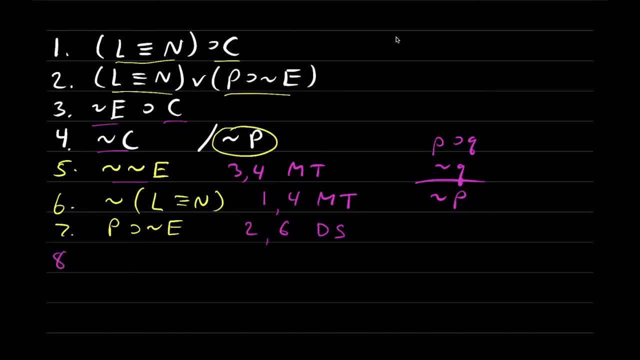 That's what we got. on line seven: P implies not E. Let's add a new line, line eight: Okay, So our new expression on line seven: P implies not E. that's a conditional. if P, then not E. but on line five, we know that not E is false. we have not not E or the negation of not E. 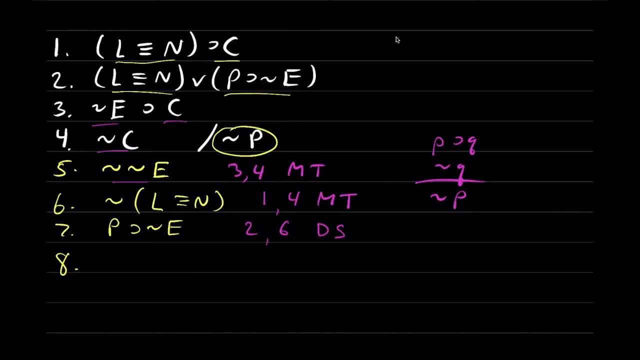 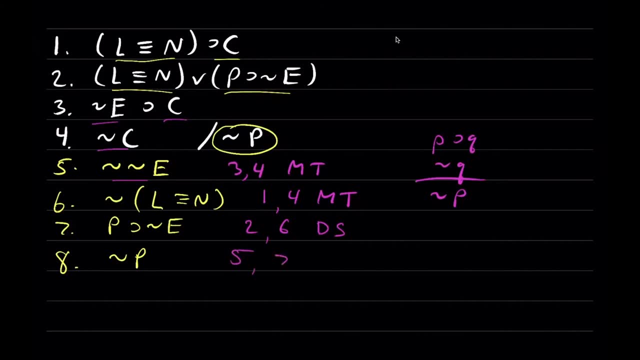 So from that we can conclude the negation of this antecedent in line seven, and that will give us not P, And that will follow from line five And line seven by modus tollens And we're done. We've got not P on its own line. So we've shown that that argument is a valid argument And it only took four steps. 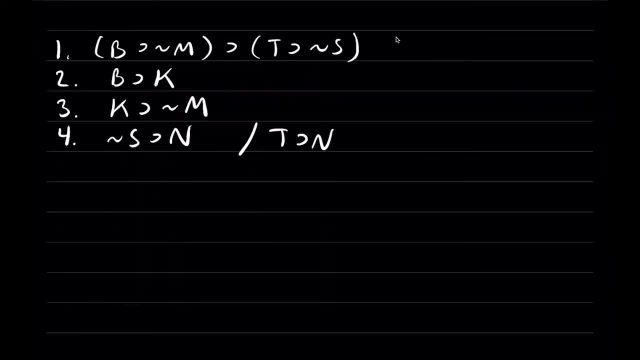 Okay, Let's do another one. This one's going to look a little scary, but don't be intimidated by it. The first premise says: if B implies not M, right, if all of this in parentheses, then T implies not S. Line two says B implies K, or if B, then K. Line three says K implies not M. Line four says that if not S, then N, And we're trying to show this conclusion: T implies N. So let's dive in. 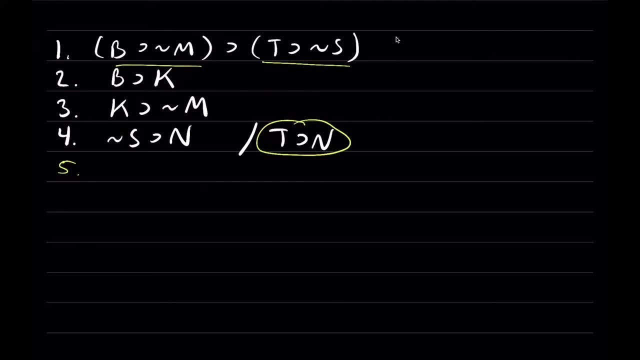 So right off the bat I noticed that on lines two and three we've got two conditionals and the antecedent is false. So we've got B implies K on line two, but line three tells us that K implies not M. So from that we know that B has to imply not M. 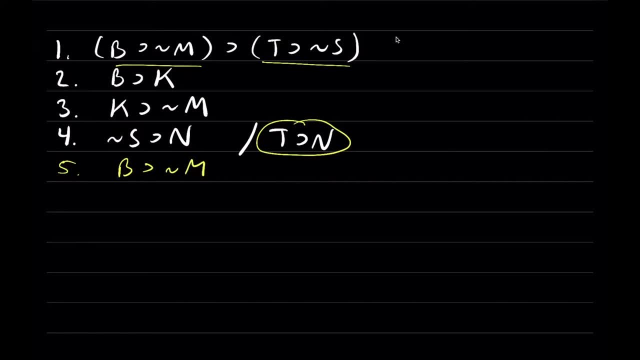 Again, just to talk through the reasoning. line two says if B then K, but line three says: but if K is true, then not M is true. So if B, then not M. And that's going to follow from lines two and three by hypothetical syllogism. 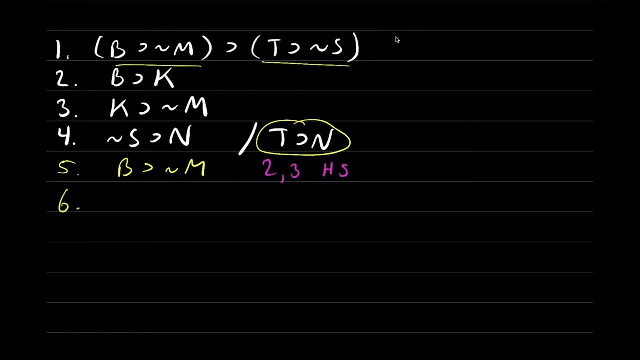 Hs. Okay, Now notice that line five is the antecedent of this conditional on line one. Line one said: if B implies not M, then we get that expression on the right in parentheses. And line five: we know that B implies not M. 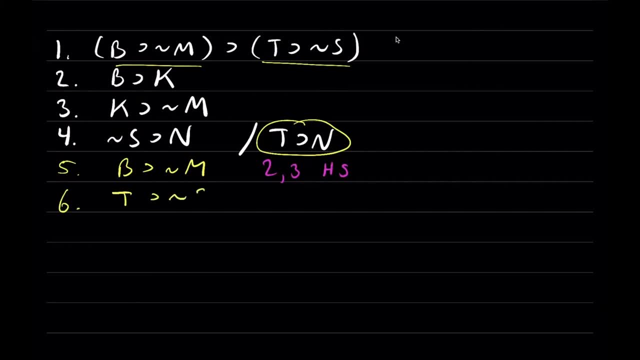 So from that we can get T implies not S, which is the expression in parentheses way up here in line one. And that would follow now from line one And line five by modus ponens. Okay, Excuse me. So we're trying to get T implies N. That's the goal, That's the conclusion that we're trying to show follows from these premises. 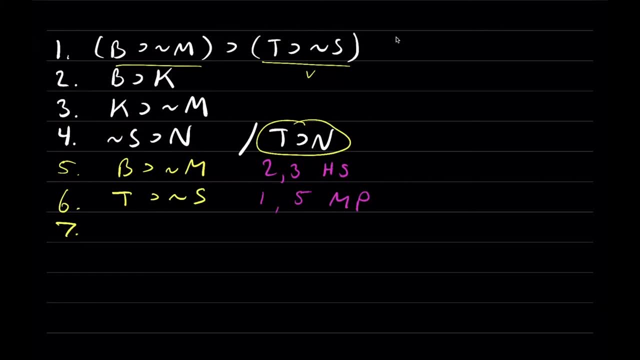 The next thing I noticed is that we have two conditionals here where the antecedent of one is the consequent of the other. I'm going to just circle them here: Line four and line six. Line six is the antecedent of one. 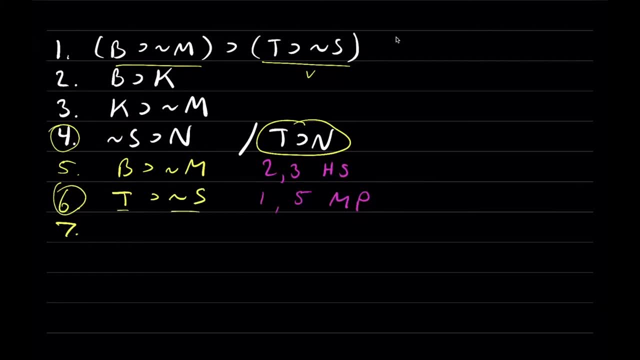 Line six says that if T is true, then not S has to be the case. But line four says that if not S is the case, we get N. From those two premises you can conclude: if T, then N, And that's going to follow from lines four and line six by hypothetical syllogism Hs And we're done. 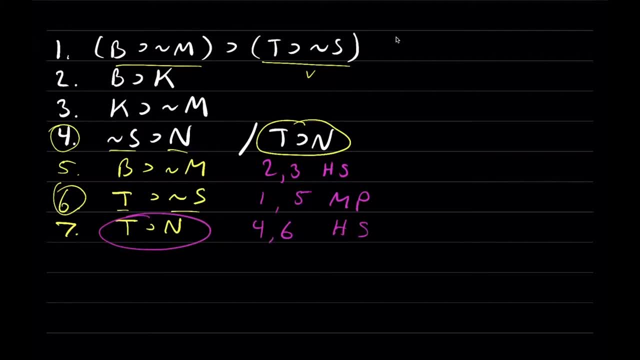 Once you get the conclusion on its own line, you've shown that the argument is valid. And here it only took three additional lines. So even though we had a fairly scary-looking conclusion, we're done. So, even though we had a fairly scary-looking first premise, notice that it didn't take much to power through this and show that conclusion followed. 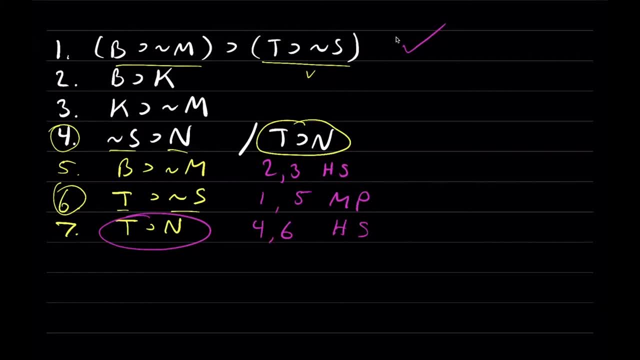 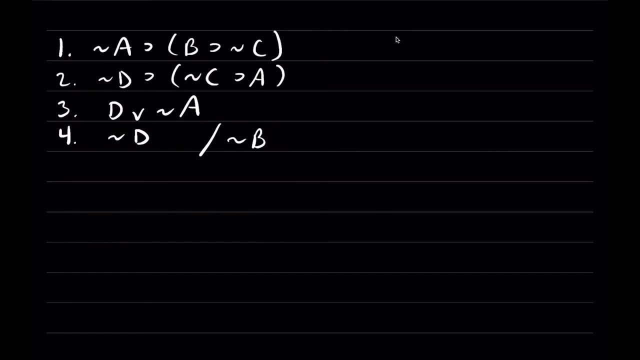 This is the power of natural deduction for showing that arguments are valid. Okay, let's do a few more. Okay, this argument. we've got four premises. The first one says: if not A, then B implies not C. Line two says: if not D, then not C implies A. Line three tells us that either D or N is the case. 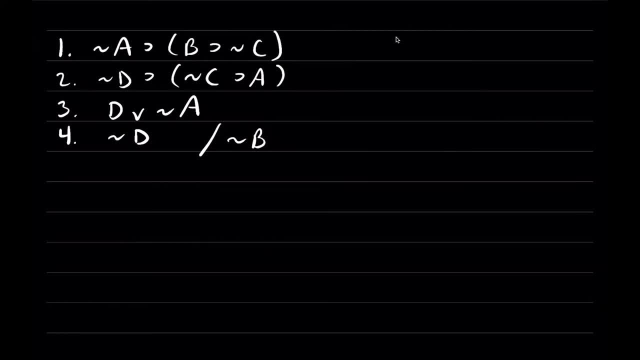 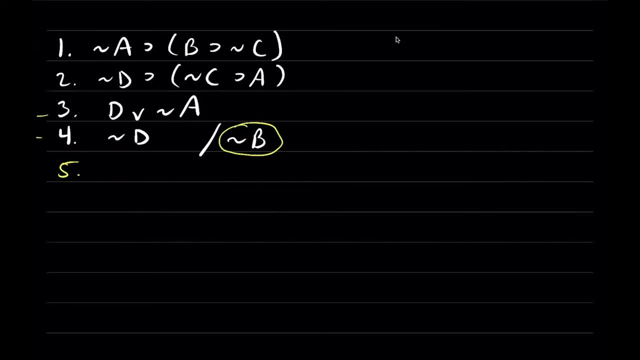 Line three tells us that either D or N is the case. Next, you might notice that lines three and four- right here and right here- match the form for disjunctive syllogism. So we could do a disjunctive syllogism right off the bat. 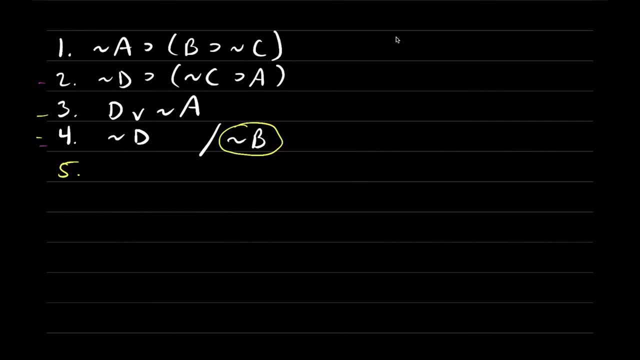 But you might also notice that line two and line four match the form for modus ponens, So you could do a modus ponens step. You will probably have to do both of those steps, So it doesn't really matter where you start. 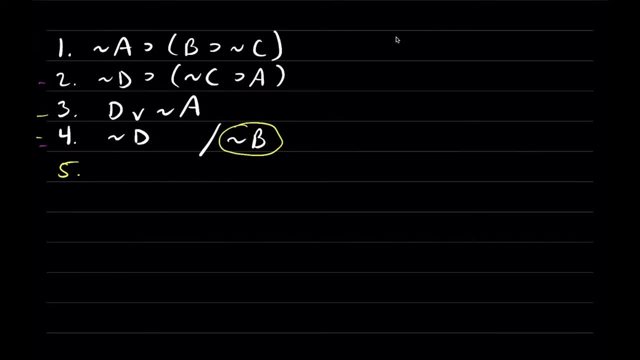 I like to start with the things that look easiest. honestly, Sometimes that can actually make the proof a little longer. Sometimes- Or you don't want to- you can actually take a shorter path to getting the conclusion by starting with something that looks a little more counterintuitive. But I like proofs to be easy to understand, So I want to take 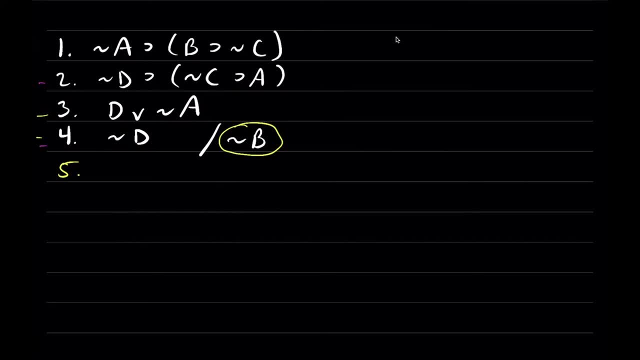 the. what I want to do is do the rule. that is the simplest rule I can do, And that's again later in the course. that's actually not going to help you. You want to be a bit more strategic, But for now let's just do the things that are really easy to do. So lines three and four, we said match. 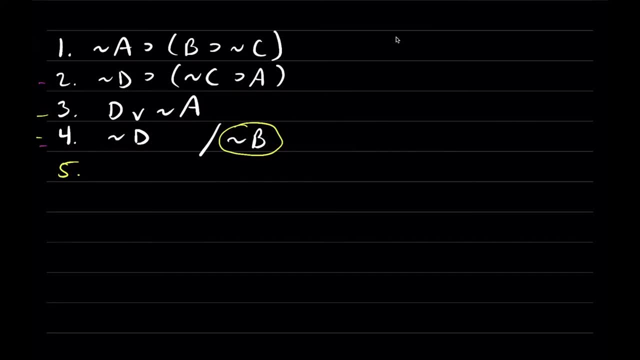 the form for disjunctive syllogism. Line three says that either D or not A, but line four told us that D is false. So from that we know that not A has to be the case, And that would follow. 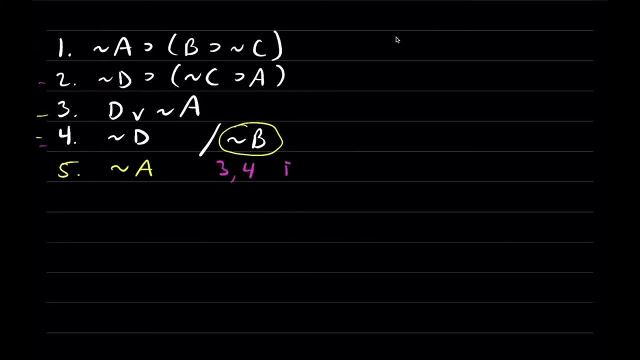 from lines three and four by disjunctive syllogism, And a moment ago we said that lines two and four match the pattern for modus ponens, So let's do that step next and get that out of the way. Line two says: if not D, then all of that expression in parentheses, not C. 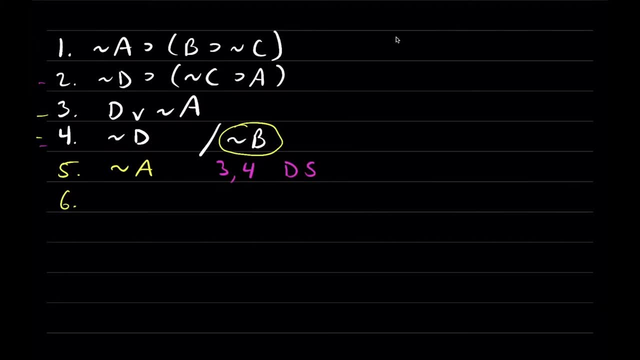 implies A. Line four says not D is actually the case, So we get not C implies A. That expression up here in line two inside parentheses, And that follows now from line two and line four by modus ponens. Okay, line seven: Notice now that we have the antecedent of that. 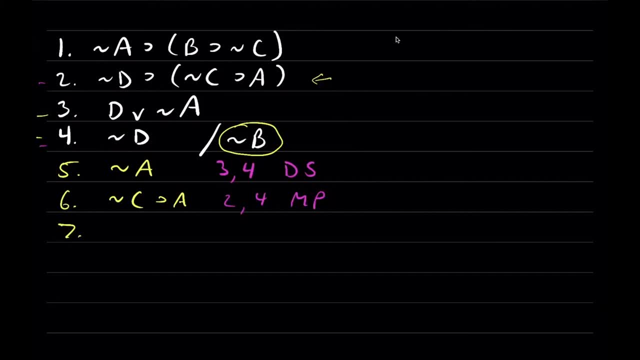 conditional in line one. Line one says: if not A, then B implies not C. Five says that not A is the case, So we get: B implies not C. That would follow from line one and line four by modus ponens. 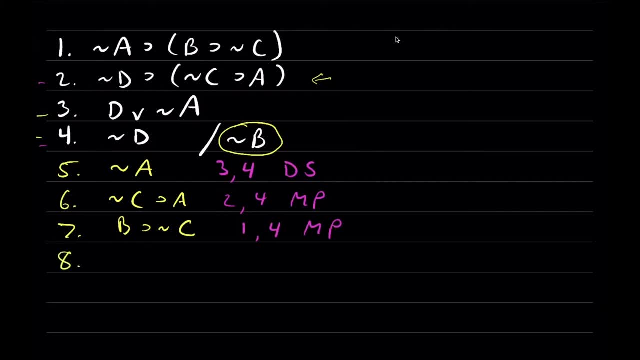 Okay, Now notice line six and seven. Again you've got two conditionals and the consequent of one is the antecedent of the other. Line seven says B implies not C. but line six tells us that not C in turn implies A. We know from that that B implies A. 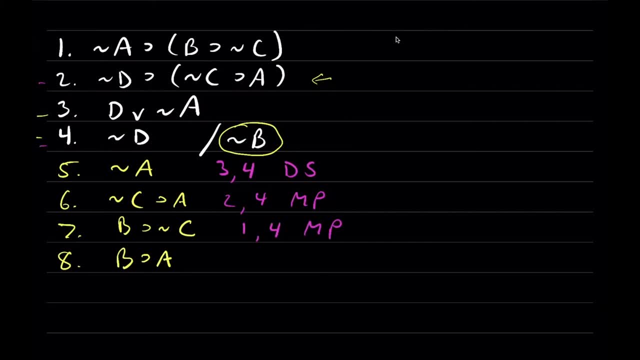 And that would follow from line six and seven by hypothetical syllogism. HS Always keep the goal in mind. We're trying to show not B, So the second we get not B on its own line using a valid inference rule. we're done. 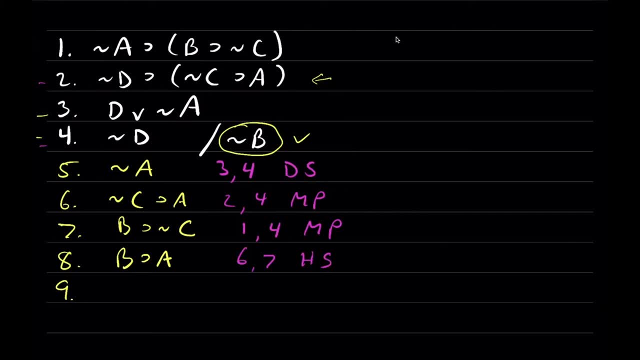 Okay, Okay, Okay, Okay. So line eight says B implies A, but in line five we know that A is false And that tells us that B has to be false according to modus ponens. So on line nine we get not B, which is our conclusion. So this is going to be the last line. 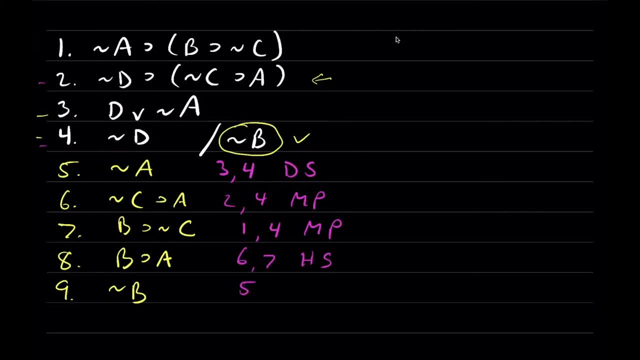 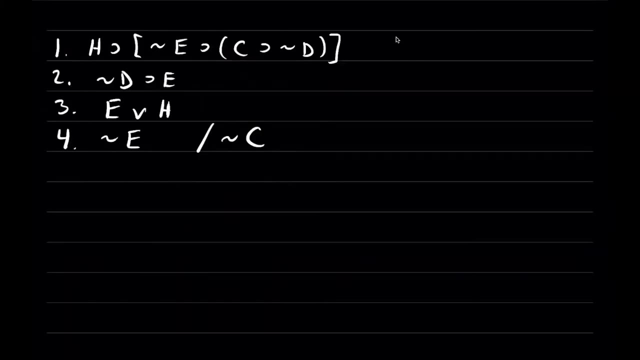 This is going to follow from line five and line eight by modus ponens, And we are done. It only took five additional lines. Okay, Let's move on. Let's move on. I think you can see these are a lot more fun and easier to do and take a lot less ink than doing a truth table. 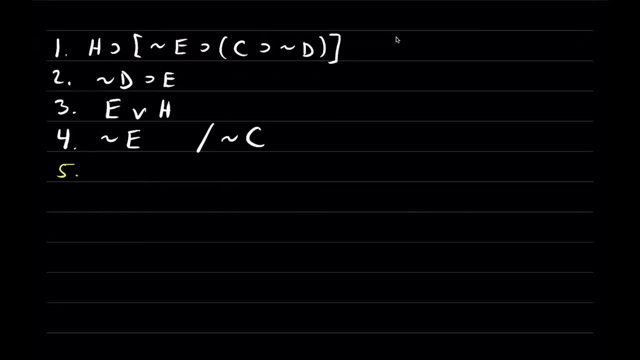 Okay, So we've got four premises. H implies this long expression inside the brackets, And it's helpful not even to worry about that. Notice that this is still a conditional. If H, then something in brackets that we don't have to worry about yet. 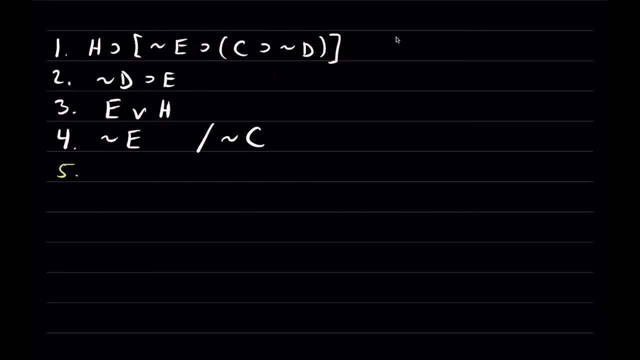 Line two says: not D implies E. Line three says either E or H. Line four tells us that E is false And we're trying to show the conclusion, not C. Okay, There are a couple places we could start. Notice that in line two we have a conditional: not D implies E. 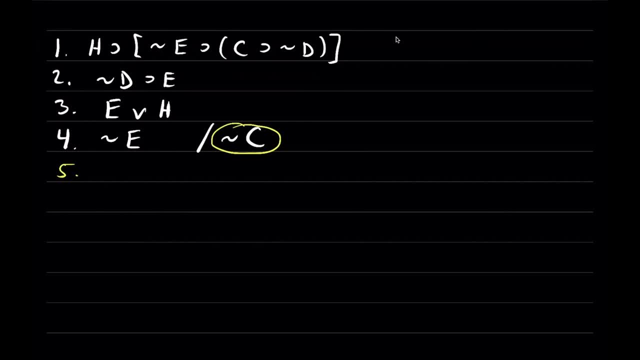 And we know that the consequence of that conditional E is false. That's what four tells us. In line three we also have E or H And we know E is false. Line four tells us that Do a modus tollens step with lines two and four. 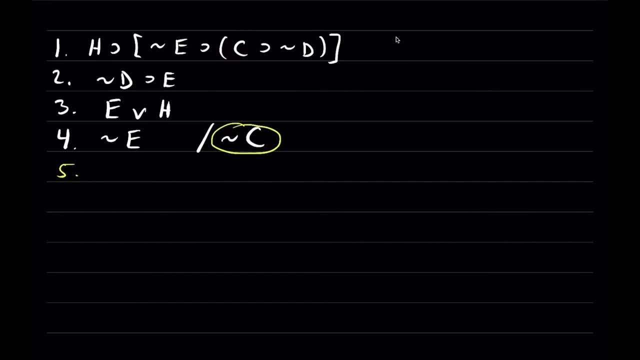 Or we could start with a disjunctive syllogism in lines three or four. Let's start with lines two and four. So line two tells us not D implies E. Four tells us that the consequence of that conditional E is false. 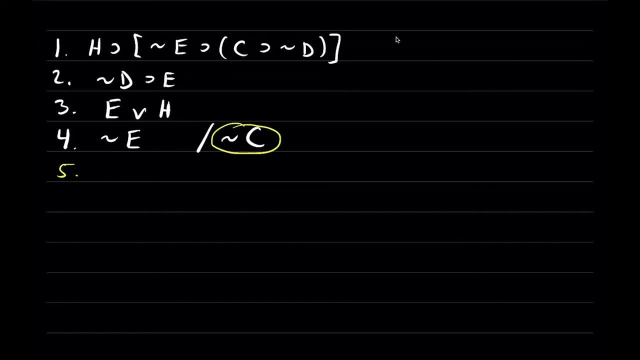 So we know that the antecedent has to be false. And here you've got to be really careful. The antecedent is not D, And for that to be false, that would be not not D. Two tildes back to back. 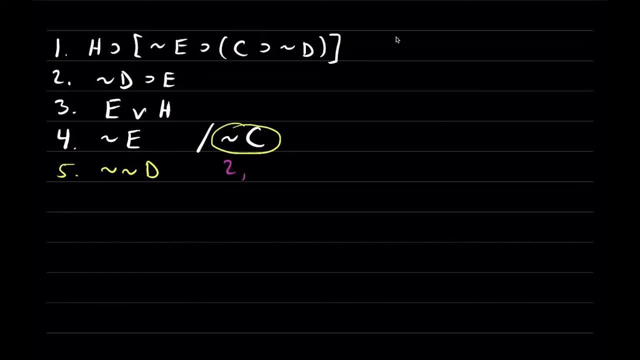 We're going to follow now from lines two and four by modus tollens, M, T. Okay, Let's do that disjunctive syllogism step we mentioned. So on lines three and four. line three is either E or H. 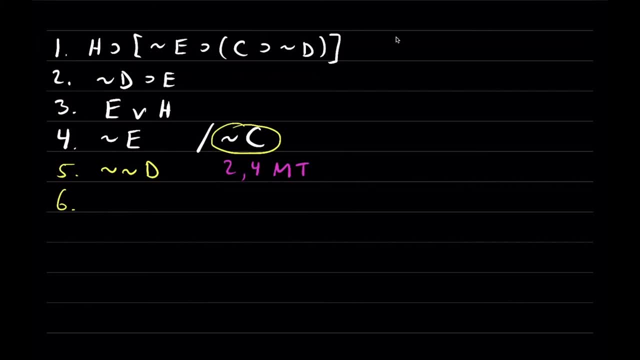 It's a disjunction. Line four tells us that E is false, So we know H has to be true And that's going to follow from lines three and four by disjunctive syllogism: D S Okay. 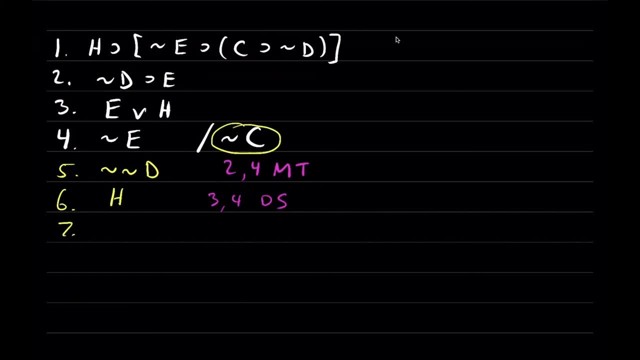 Line seven. Now here's where we're going to use that very scary-looking first premise, which isn't as scary as it looks. Line one says: if H, then that entire expression in brackets follows, And we don't want to worry about what that expression is yet. 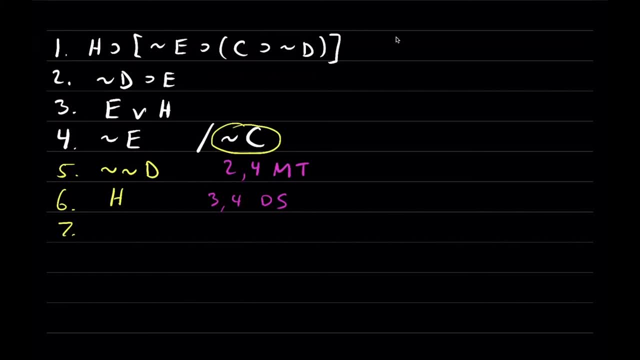 We just know that if H is true, we get that expression in brackets, And line six tells us that H is true. So we know that that entire expression inside the brackets has to be true. All of this right here that I'm going to indicate with the yellow line. 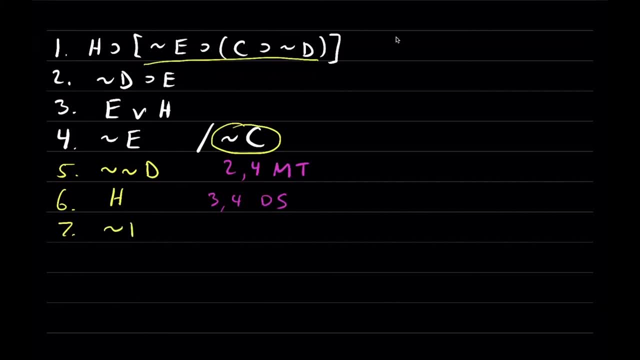 So in line seven I'm going to get that entire bracketed expression. Not E implies with parentheses here, Don't miss anything. C implies, not D, All of that And that's going to follow now from line one and line six by modus ponens. 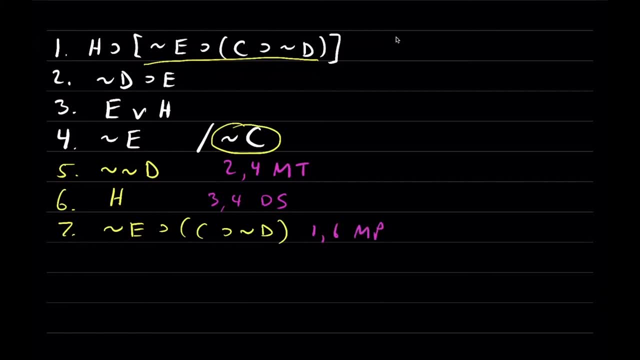 So even though that's a fairly scary-looking expression, it still has the form. P implies Q, P therefore Q. It just so happens here that Q stands for this entire expression in the brackets. That's what we got on line seven, Q on its own line. 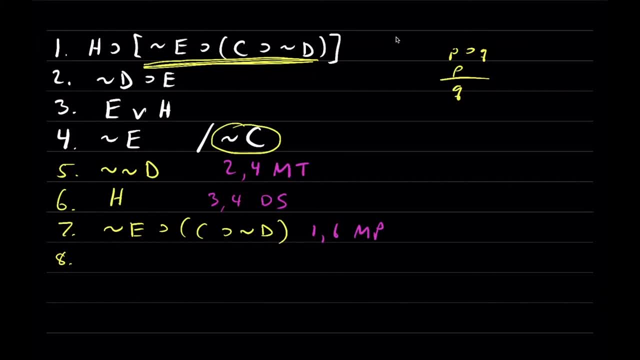 Okay, Line eight. The next thing I notice is that seven is a conditional. If not E, then C implies not D. If not E, then that expression inside parentheses, And we have not E on line four, And so by modus ponens we can get that C implies not D. 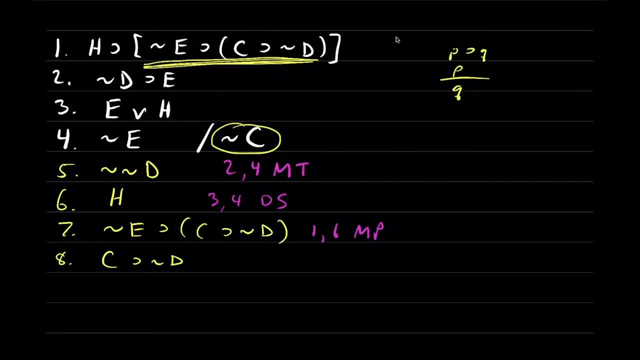 And that's going to follow now from line four and line seven by modus ponens. So again, notice that there's nothing to tell me what I have to do next. You have to rely on your pattern recognition skills to be able to identify these argument patterns. 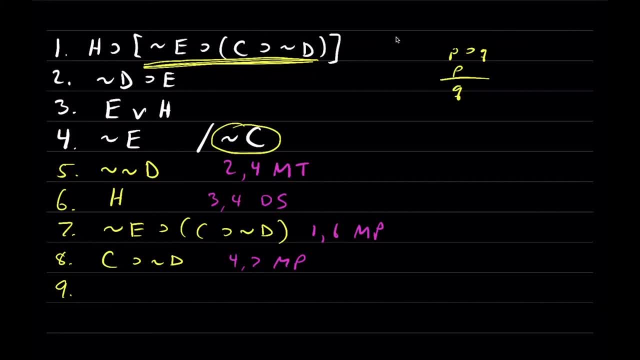 inside the statements that you're given, And that just takes practice. So please, please, please, do plenty of practice. Even do extra. you know, redo the ones I've done in the video, Do the ones in your homework, Do the sample exercises from section 7.1 of your textbook. 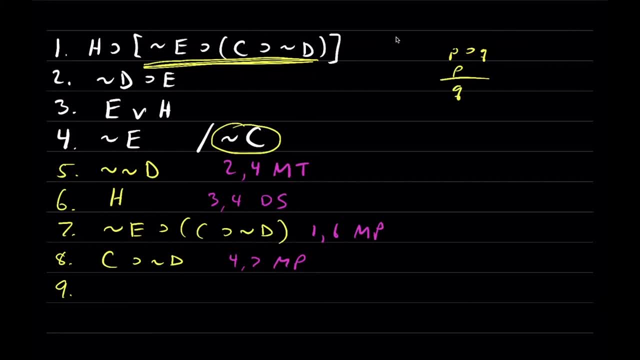 Get as much practice as you can on this. As you can see, any given proof doesn't take very long. Your homework probably won't take you very long this week, But get lots of extra practice on this, Okay. The next thing I notice: 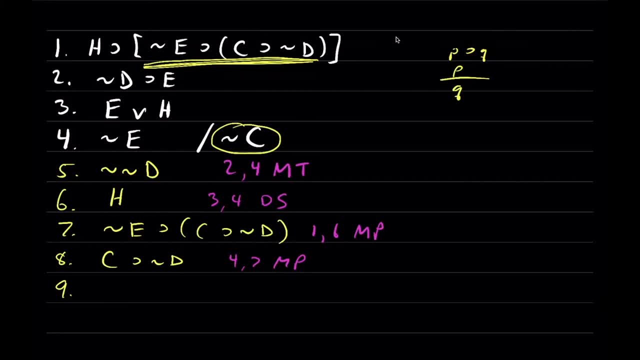 is that on line eight we've got a conditional. C implies not D, But number five tells us that not D is false. We have not not D. From that we know that the antecedent of the conditional in line eight 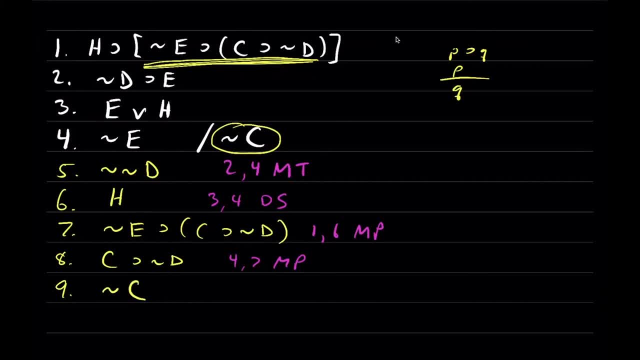 C has to be false or not C, And that would follow now from line five and line eight by modus tollens And we're done Once we've got not C on its own line. that's the conclusion we were trying to get. 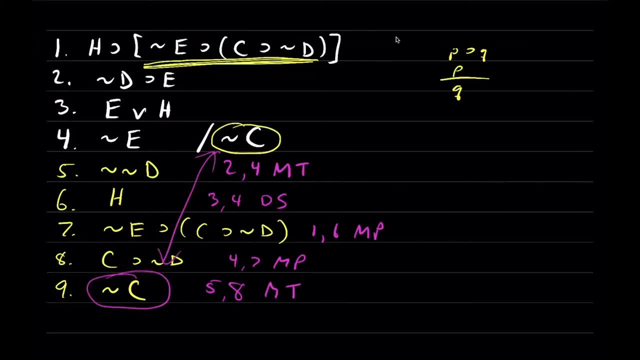 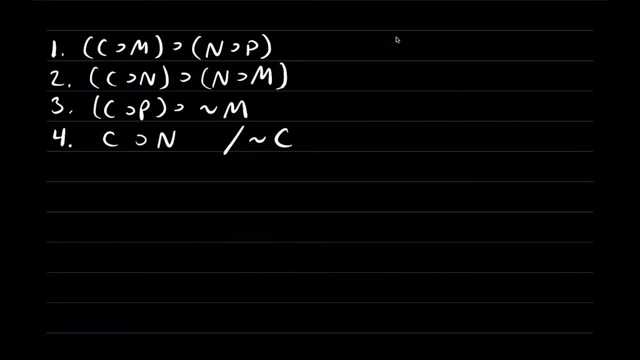 We're going to show followed. We've finished the proof and we've shown that argument is valid. Didn't take very many steps. Okay, As we keep going through the rest of the exercises I have for you guys, these are going to get a little sort of bigger, longer, scarier looking. 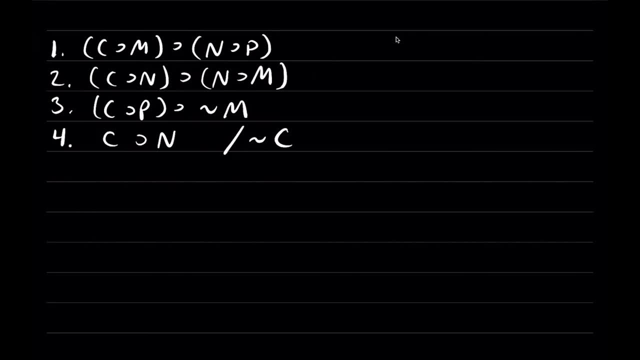 But if you break them down as I'm doing here, you can see that they're not terribly complicated. Okay, Line five. Well, let me run through the premises first, like I've done before. At a certain point, you know, you need to be able to identify these yourself. 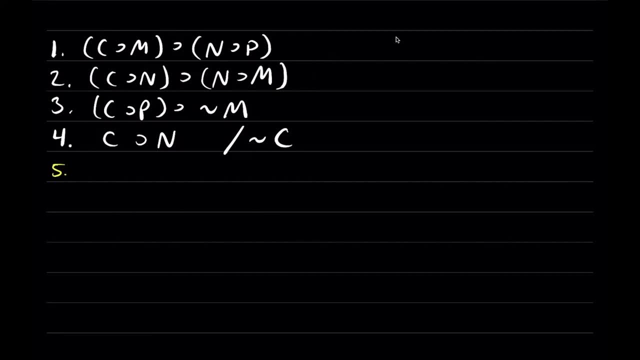 And I'm reading each premise out loud to you to reinforce what I notice when I see these statements. So line one is a conditional. It says: if this expression in parentheses, if C, implies M, then this other expression in parentheses, N, implies P. 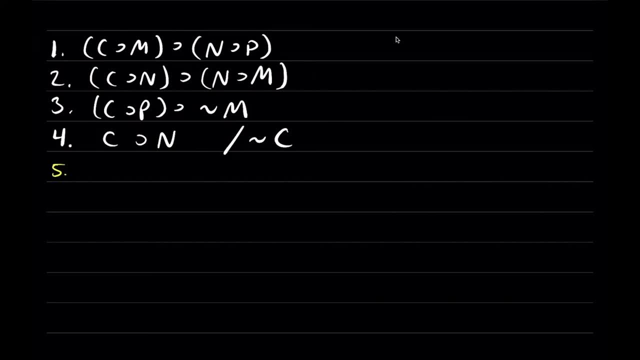 Line two says that if C implies N, be careful, here we have M's and N's. That's a little almost visually cluttery. So if C implies N, then this other expression in parentheses on the right, N, implies M. On line three we've got a conditional. 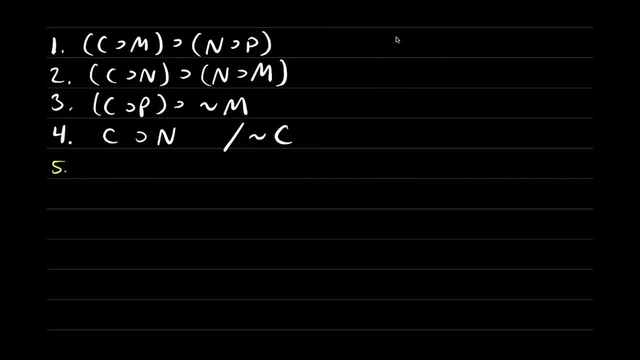 If C implies P, then make sure you notice the main operator there, then not M. Line four says that C implies N and we're trying to show from that that C is- excuse me, C is false. Okay, Let's dive in. 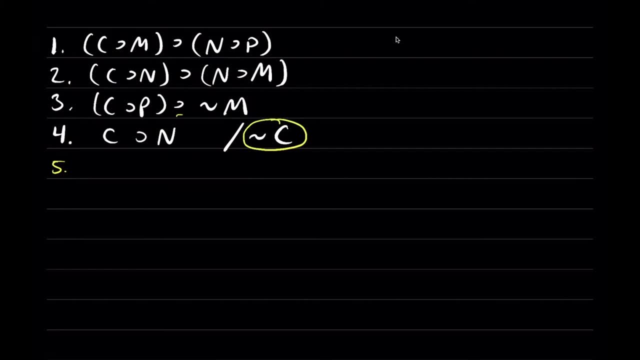 The thing I noticed right off the bat is that line four is the antecedent of this conditional in line one, right, Or, excuse me, in line two. Line two says: if C implies N, then we get this expression in parentheses on the right: N implies M. 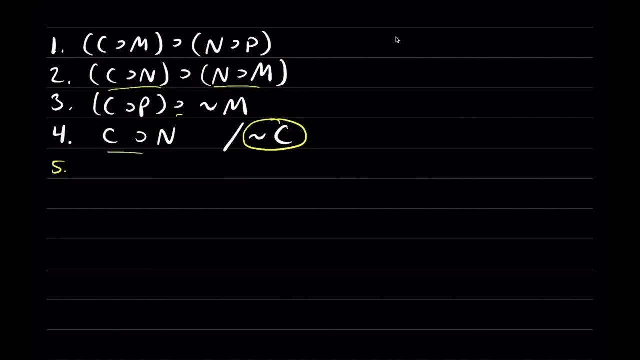 Line four says that C does imply N. so we know from that that N implies M, And that's going to follow now from line two and line four by modus ponens. And again, if you need to review the rules, pause the video. 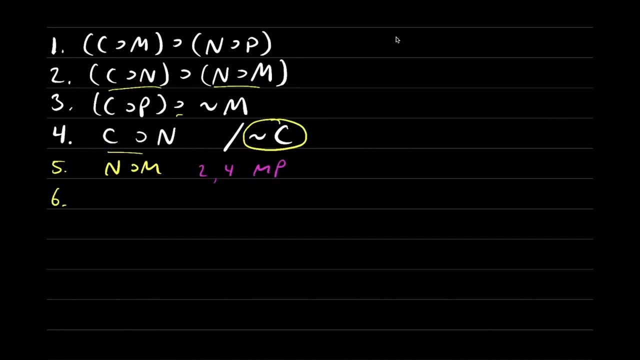 crack open the textbook and look at what modus ponens does. look at line two and line four and you should be able to see the pattern inside those statements. Okay, The next thing I notice is that in lines four and five you've got two conditionals. 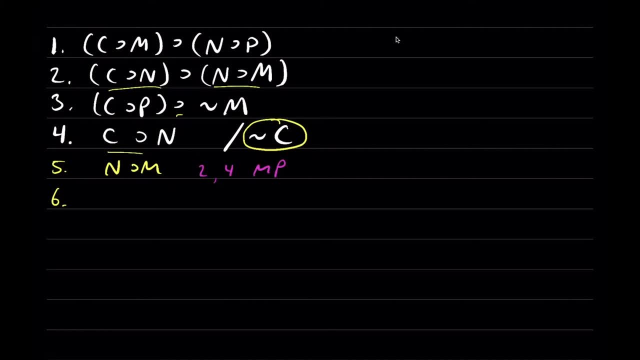 and again the consequent of one is the antecedent of the other. Line four says: if C then N. Line five says: but if N then M. So we know from that that C implies M And that's going to follow from line four and line five by hypothetical syllogism HS. 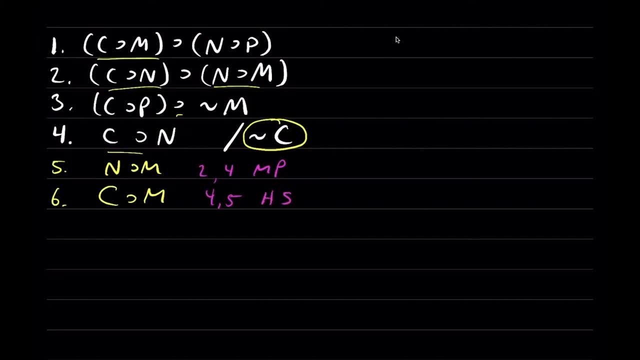 But once we know that C implies M, that's the antecedent of this conditional in line one. So from that we know that N implies P, the consequent of that conditional in line one. And that's going to follow from line one and line six by modus ponens. 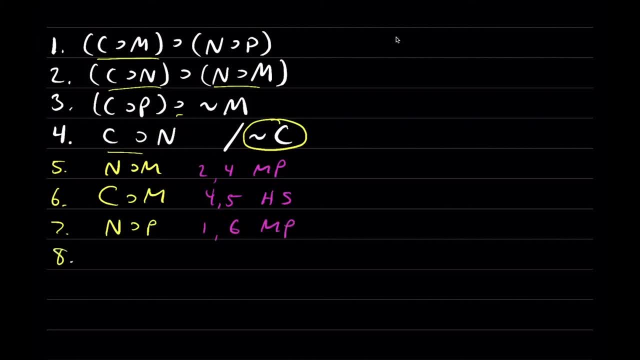 Okay. Next line, line eight: Okay, The next thing I notice is that on line four and line seven we've got two conditionals Again. the consequent of one is the antecedent of the other. Line four says: if C, then N. 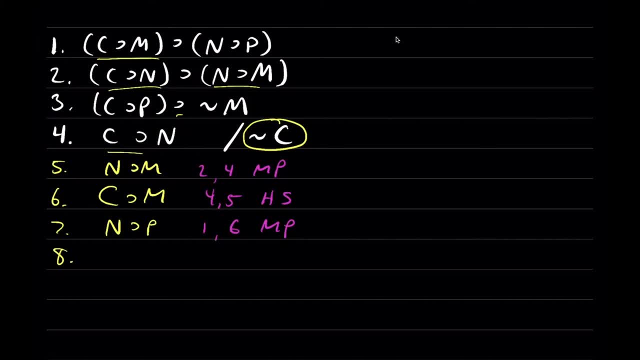 Line seven says: if N, then P. From that it follows that if C, then P, And that would follow from line four and line seven by modus ponens. Okay, Next line, line eight: Okay, The next thing I notice is that on line four and line seven we've got two conditionals. 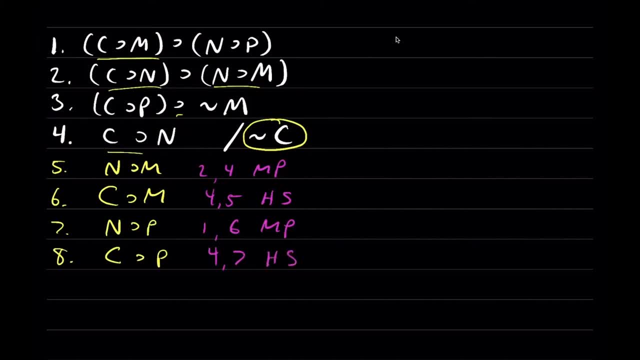 Again, the consequent of one is the antecedent of a hypothetical syllogism. Okay, But that gives us the antecedent of this conditional in line three. if C, then P. If that is the case, you get not M. 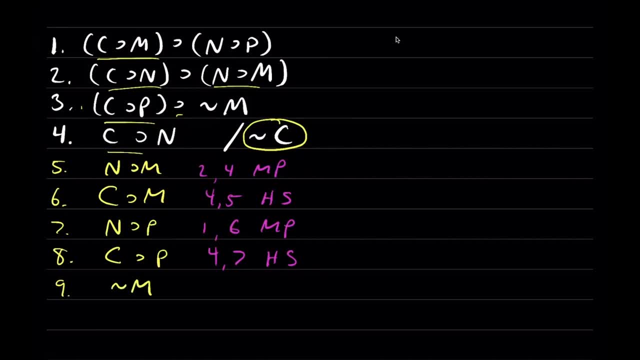 So on the next line we can write not M, And that's going to follow now from line three and line eight by modus ponens, And that's going to follow now from line nine by modus ponens. Okay, So we've got not C on line 10.. 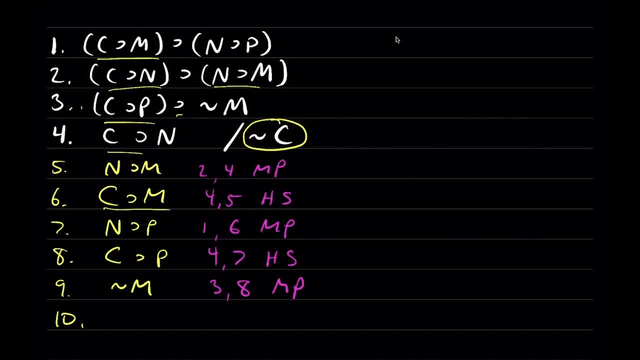 Remember, we're trying to get not C on its own, And in line six we've got a conditional: If C, then M. Line nine tells us that M is false. We know from that that C has to be false And that's going to follow now from line six and line nine by modus ponens: M, T. 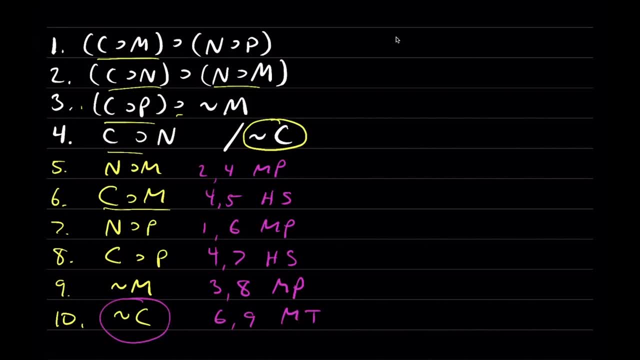 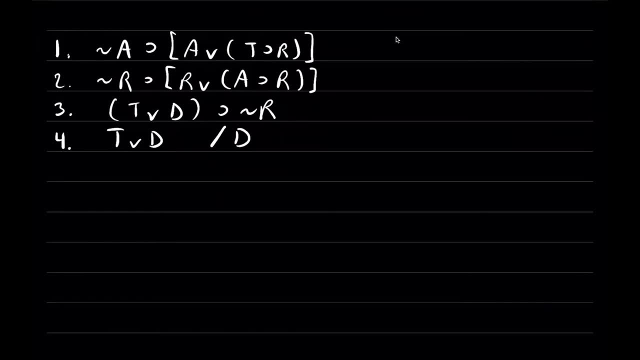 And we're done. We've got not C on its own line. Okay, I've got one more for you guys, And then I will give you your time back And you can get lots and lots of practice doing proofs on your homework exercises for the week. 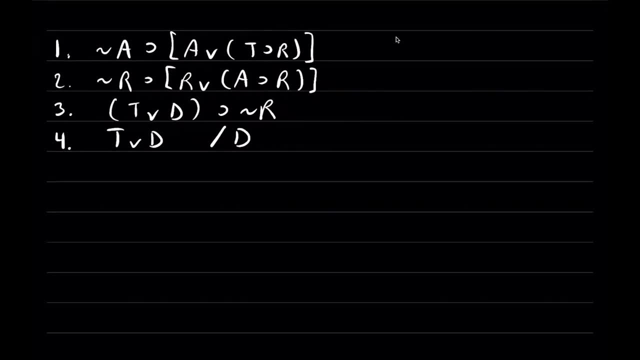 We have four premises. Line one says that if not A, then that entire bracketed expression on the right. Line two says: if not R, then that entire bracketed expression on the right. Don't worry about what those are. yet. Line three says that if T or D, then not R. 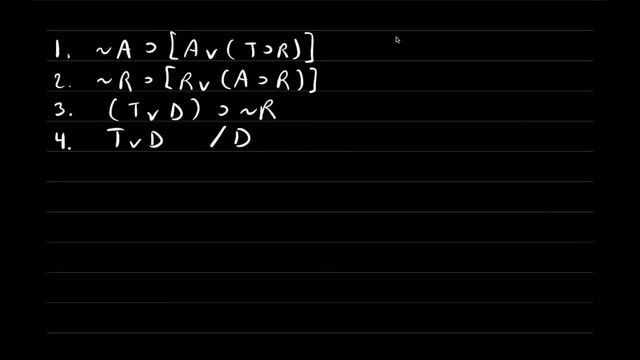 Line four says T or D is actually the case And we're trying to show that D follows from that. So let's dive in Line five. The very first thing I notice is that line four, T or D is the antecedent of the conditional here in line three. 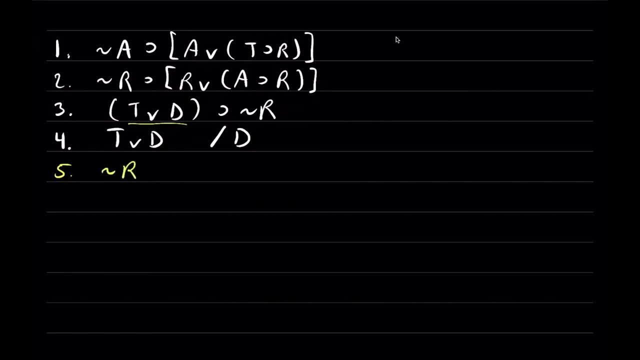 So from that we know not R has to be the case, And that's going to follow now from line three and line four by modus ponens. Okay, Next line Line nine, Line six: Once we have not R, that's the antecedent of the conditional in line two, right here. 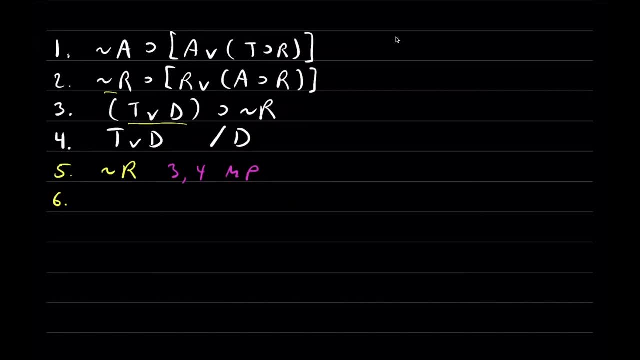 So we know that that bracketed expression R or A implies R. inside brackets has to be true R or in parentheses now, A implies R And that's going to follow from line two and line five by modus ponens. But that expression we got on line six, R or A implies R, is a disjunction. 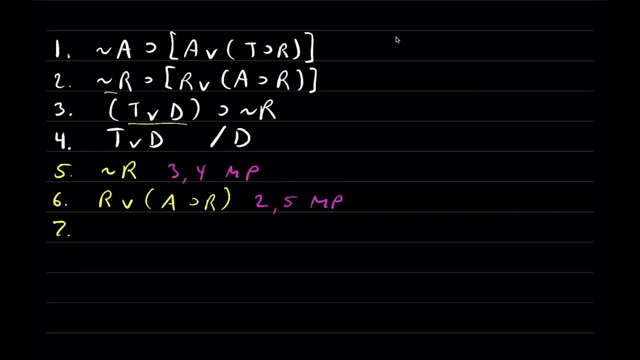 It says either R is the case or that expression in parentheses A implies R is the case, But line five tells us that R is false. From those two statements we know that A has to imply R, That expression in parentheses has to be true. 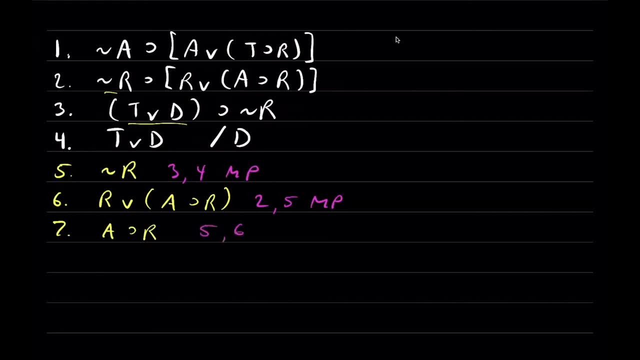 That's going to follow now from line five and line six by disjunctive syllogism. Okay, So line seven, our new line, says: if A, then R. Line five: we know that R is false. The consequent of that conditional is false. 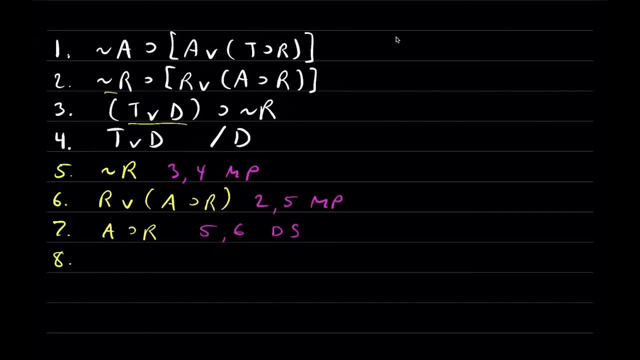 According to modus tollens, we know that the antecedent then has to be false or not, A, And that's going to follow now from line five and line seven by modus tollens. Once we know A is false, that's the antecedent of the conditional way up here in line one. 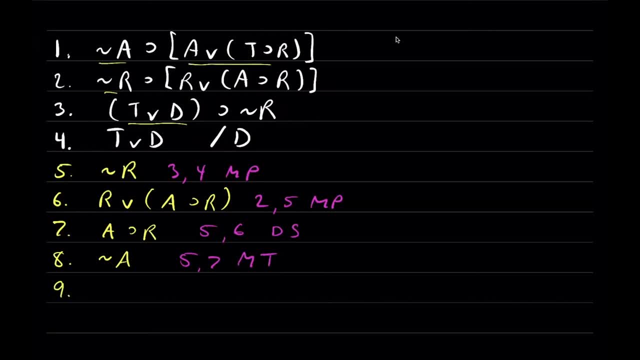 If not A, then this entire bracketed expression on the right. So we know that A or T implies R has to be the case And that's going to follow from line one and line eight by modus tollens. But that's a disjunction. 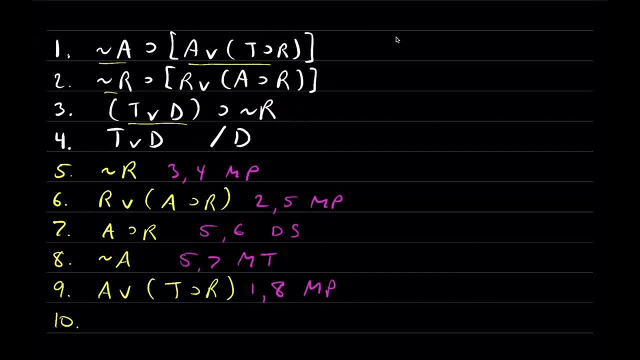 It says A or T implies R, And on line eight we know that A is false, So we know that T implies R. has to be the case that expression in parentheses That's going to follow now from line eight and line nine by disjunctive syllogism. 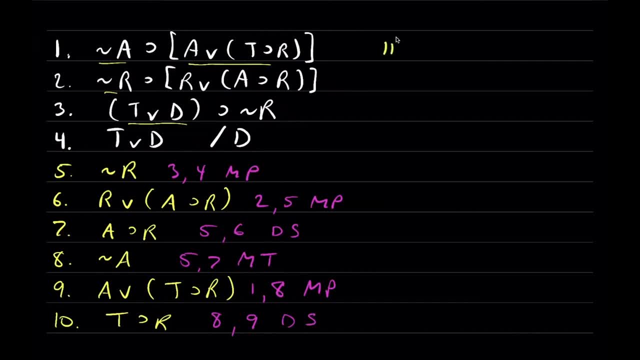 Okay, I'm going to move way up here to the top right, start a new line, line 11.. In fact, I'll draw a little dividing line here to keep this visually clear. Okay, The next thing I notice is that on line 10, we've got an if-then statement. 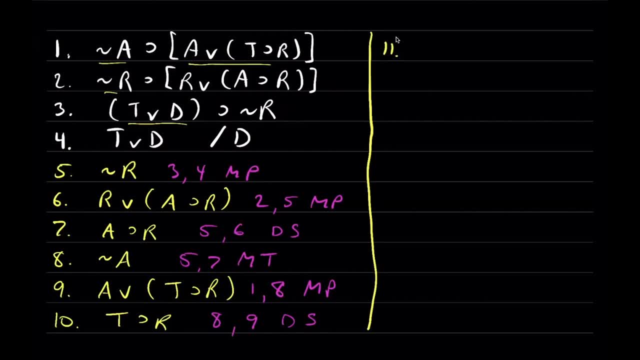 If T, then R, And way up here in line five we have not R. That's going to match the pattern for modus tollens. So we know that the antecedent of that conditional in line 10 has to be false or not. T. 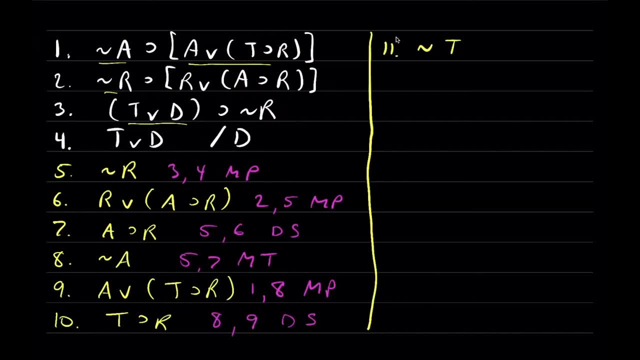 And that's going to follow now from line. Let's see It's going to follow from line five and line 10, excuse me, by modus tollens, I think we're almost done, Not quite. Excuse me. Once we have not T, we actually have the negation of one of the disjuncts way up here in line four. 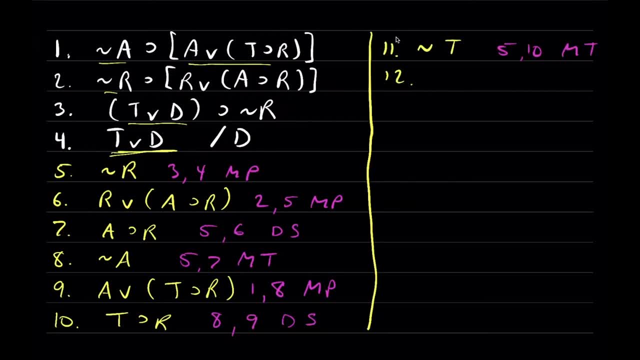 Don't forget about the statements up above that are given to you. You're allowed to use any lines that occur previously in the proof, with some exceptions that we'll talk about here in a few weeks, But for now, you're able to cite any previous lines. 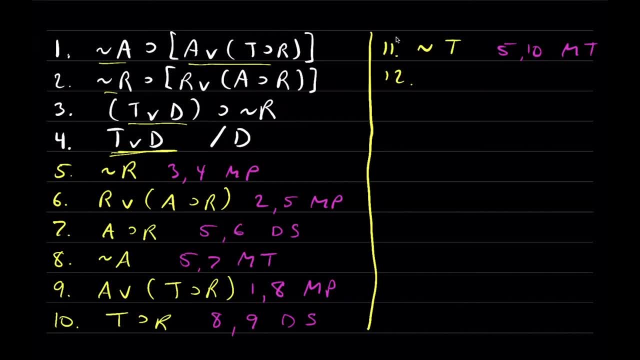 We haven't used line four yet and that should kind of stand out to you. Line four says: Line four says either T or D. Line 11, the line we just got says that T is false. So we know from those that D has to be true. 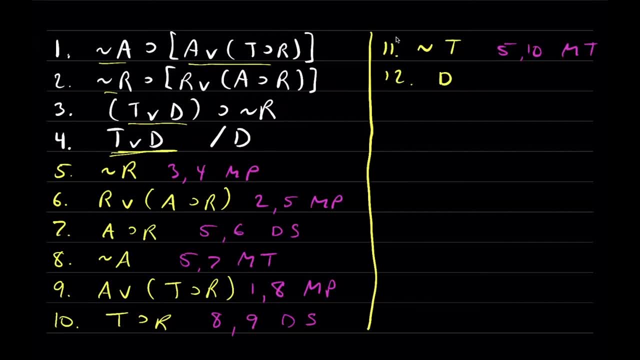 And that's going to follow now from line. Let's see What was it. Line four and line 11 by disjunctive syllogism, And notice that we're done. We were trying to show that D has to be the case. 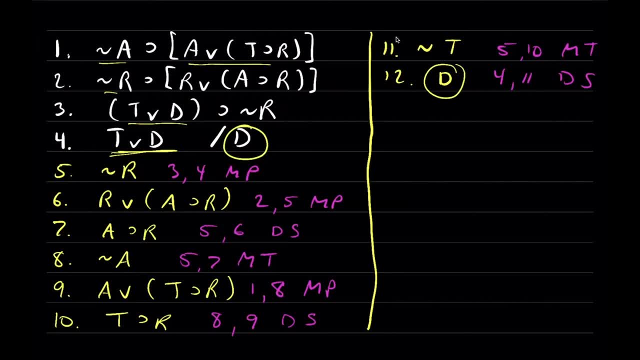 We showed that on its own line here, in line 12. And that shows that this argument is valid and it only took 12 lines. It's way faster than doing a truth table for this argument. This would have been a pretty large truth table for this argument. 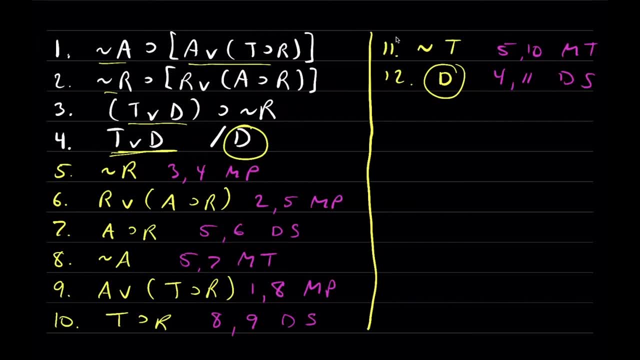 Something like: probably- Let's see How many lines A, T, R and D would have been 16 lines to do a truth table, And we did this in 12 lines, including the four that were given, So this was quite a bit more elegant. 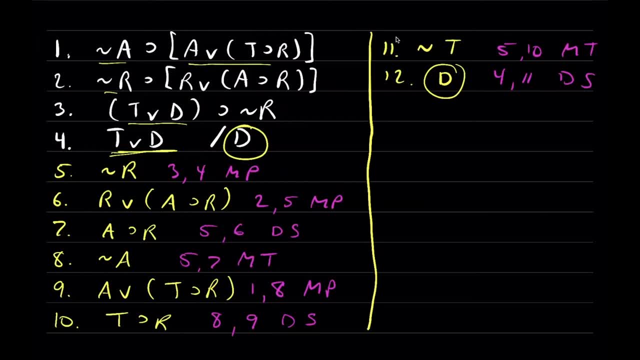 That's the last example I have for you. I want For your homework, do the odd-numbered exercises from Roman numeral. Let's see It's section 7.1.. Roman numeral, number 3.. Do all the odd exercises, all the complete proofs, in other words. 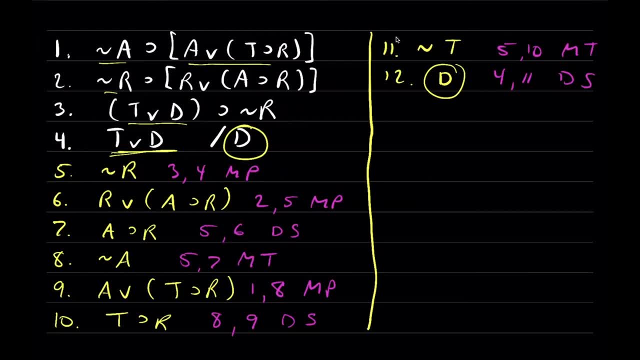 But get lots of extra practice. Redo the exercises that I did here in the video. Do the practice exercises that are given inside the textbook chapter itself. Again, let me just refresh. you know, kind of sum everything up here In an argument. you're given some number of premises and a conclusion. 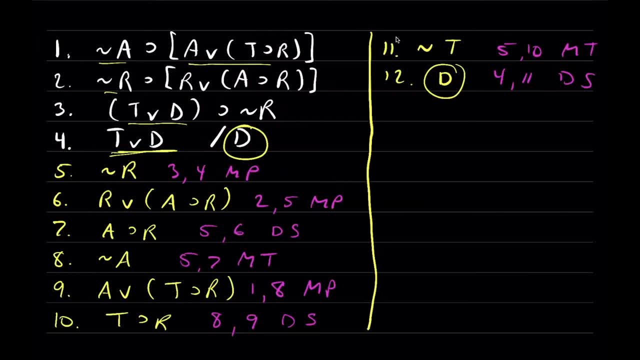 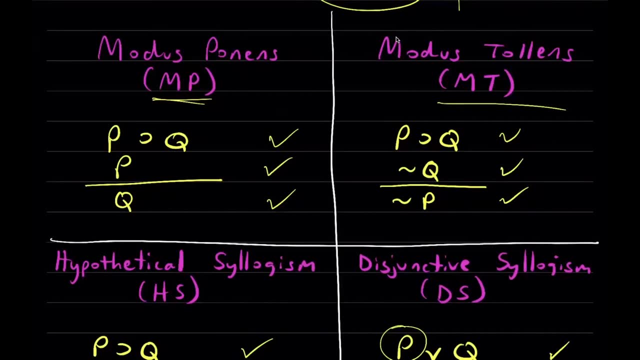 Every line of a proof needs to follow by one of these valid inference rules. I'll scroll back up here and run through the rules one more time. Modus ponens, MP, says that if P implies Q and you have P, then Q follows from that. 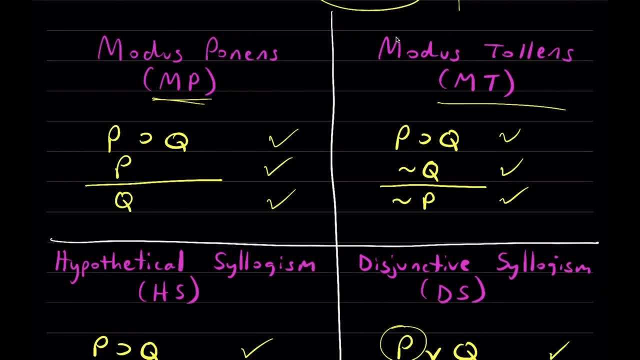 And again, P or Q here can stand for a simple statement, either you know, just a simple capital Set of capital letters, Or P or Q could stand for compound expressions in parentheses or brackets or braces, And all The entire challenge of doing proofs rests with your ability to recognize these argument patterns in compound statements. 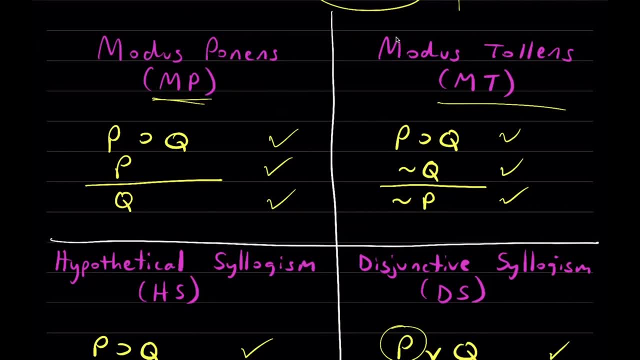 Modus tollens. MT says if P implies Q and if you have the proofs, then Q follows from that. If P implies Q and if you have the negation of the consequent not Q, you know that the negation of the antecedent, not P, has to be the case. 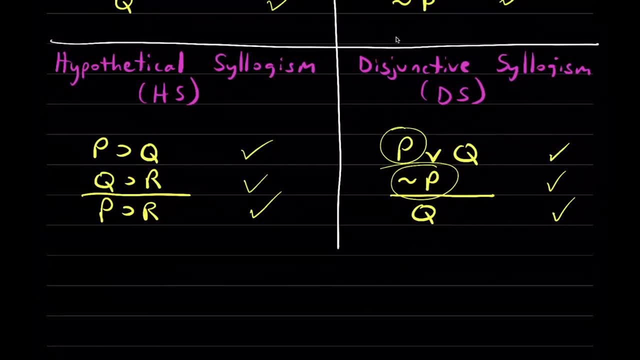 Down here hypothetical syllogism. Basically there are two conditionals where the antecedent of one is the consequent of the other. In this case, P implies Q, but Q implies R. So you know that if P is true, then R has to be true. 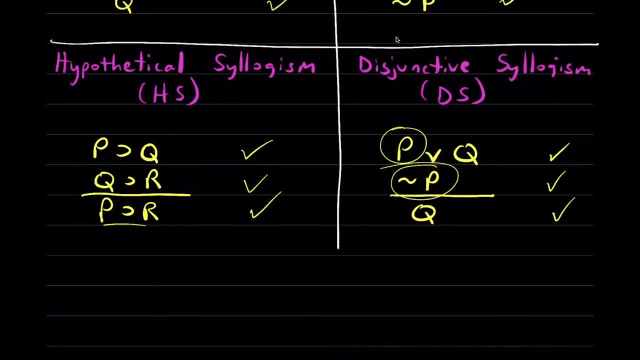 You get another conditional: P implies R. That's hypothetical syllogism, or HS. And the last argument, form disjunctive syllogism says either P or Q. But P is false. You know from that that Q has to be true. 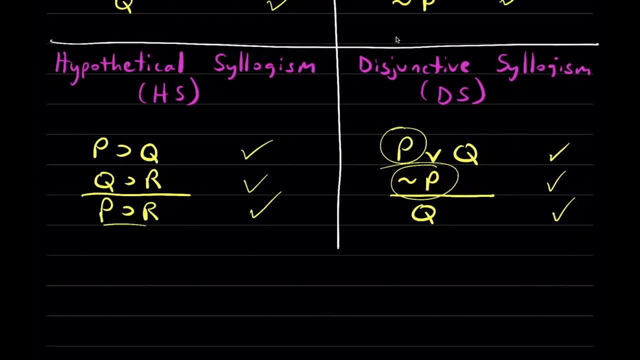 Again, P or Q could stand for atomic statements, capital letters, or they could stand for compound expressions in brackets. So again, just to summarize proofs, you're given some number of premises and a conclusion. You obviously can't cite the conclusion, because that's what you're trying to prove. 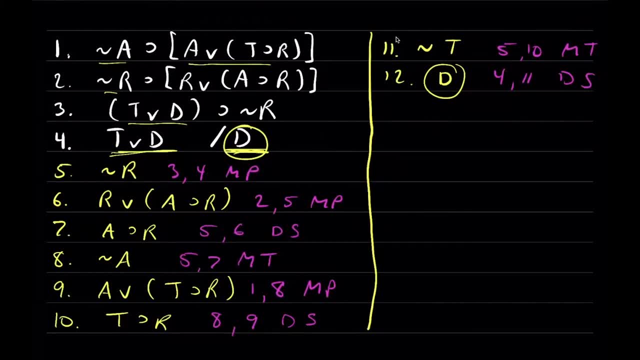 Every line needs to follow by one of the inference rules. You always cite the line numbers that the new line comes from And the rules are the same And the rule that you use to deduce that line. And if you can show that the conclusion of the argument follows on its own line, you will have shown that the argument is a valid argument. 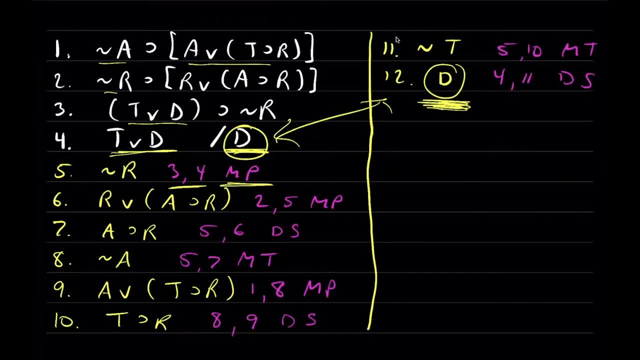 But if you're unable to show that an argument, that a conclusion follows from a set of premises, that doesn't automatically mean the argument is invalid, Because there's just no way to know. if you just weren't frankly clever enough to notice the next line, next step of the proof to do. 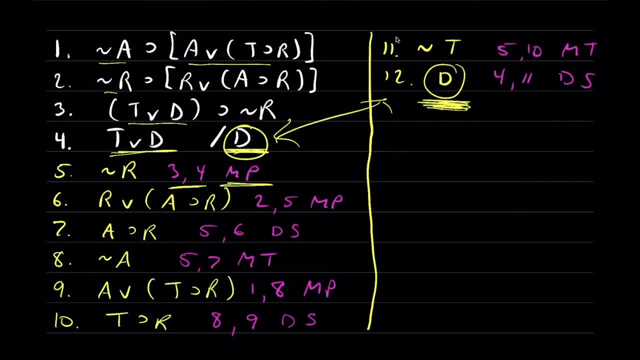 In fact it's been shown that there are some arguments that there simply is no mechanical method for evaluating the argument. In other words, you can't write a computer program to crank out a proof for any given argument. Some proofs you know kind of get you stuck in a feedback loop. 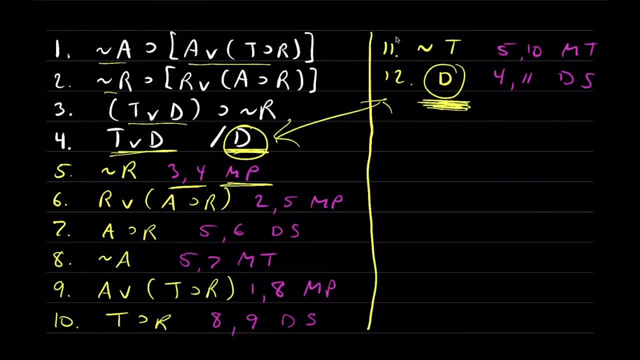 Those are well beyond what we're looking at right now. But, in other words, proofs are not a decision method. They're not 100% reliable way of taking any given argument and showing that it's valid or invalid with certainty. That's what truth tables are for.